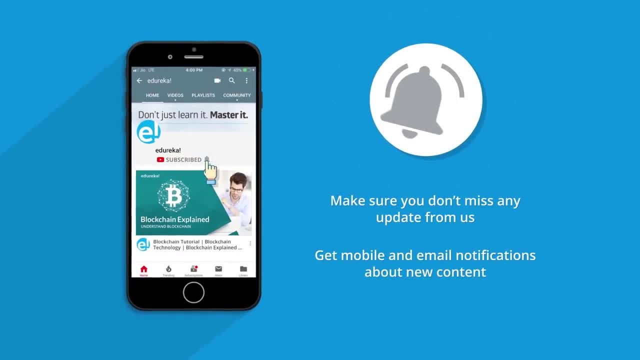 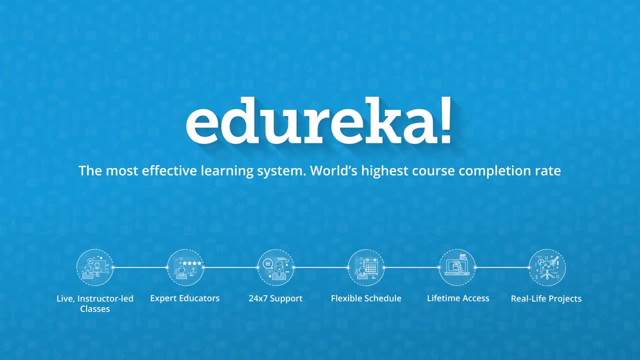 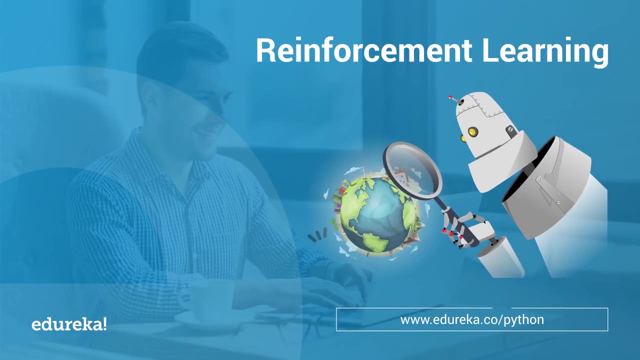 Hi everyone, this is Zuleikha from Edureka. Today's session is dedicated to reinforcement learning. Reinforcement learning is one of the types of machine learning which has been growing in the past few years. It has various applications like self-driving cars and image. 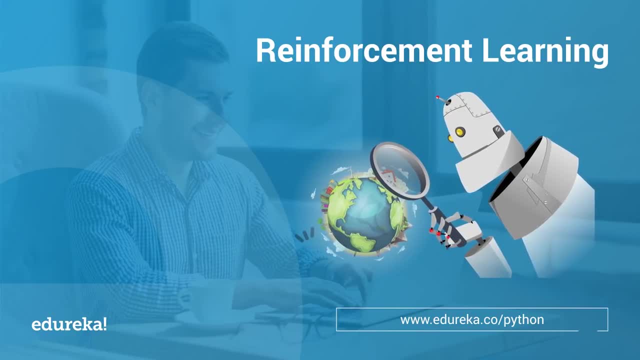 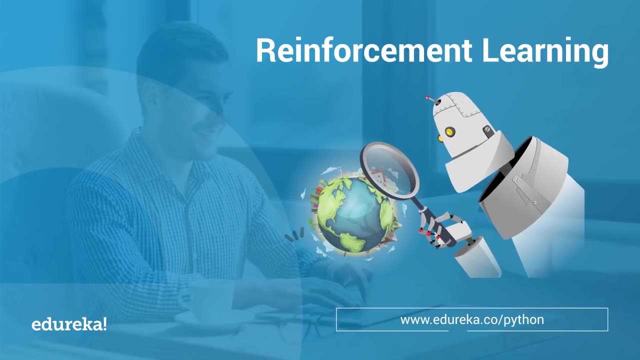 processing techniques wherein you detect objects using reinforcement learning. Reinforcement learning has become one of the most important types of machine learning in today's world, So, without any further ado, let's look at what we're going to cover today. So we're going to begin the session with an introduction to machine learning and the types of machine. 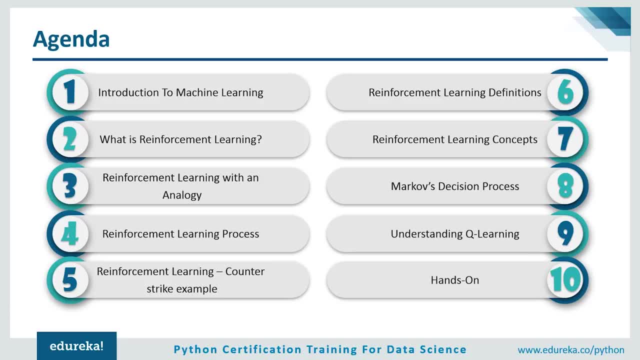 learning. After that we'll discuss reinforcement learning in depth and we'll try to understand reinforcement learning with an analogy. Once we're done with that, we'll look at the reinforcement learning process and how it works, And then we'll try to relate the reinforcement learning process with a counter-strike example. 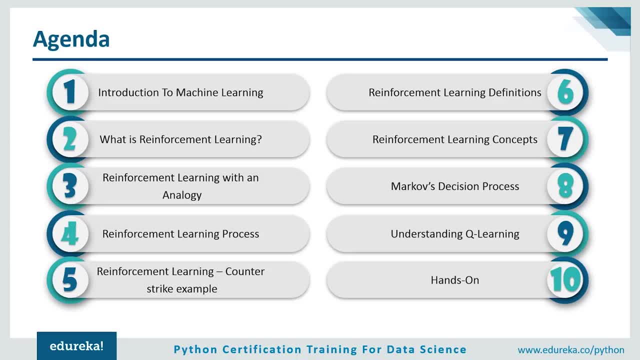 Once we're done with that, we'll look at a few reinforcement learning definitions like agent, environment, action and so on. Next we'll move on to the reinforcement learning concepts. Here we'll discuss a few concepts such as reward maximization and the concept. 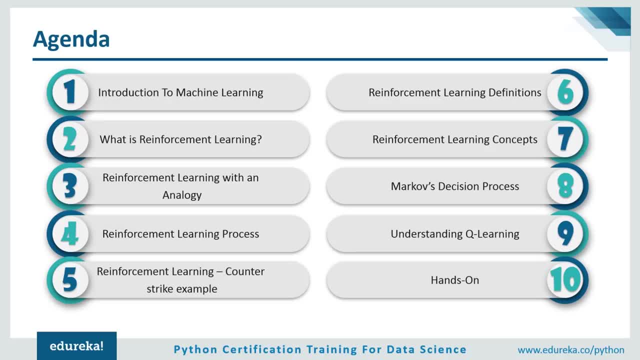 of exploration and exploitation. Then we'll finally move on to the Markov's decision process, where we'll try to understand this process with the help of a shortest path problem. Now, moving on to the demo, we'll be implementing the Q-learning algorithm. So, in order to understand the demo, we're going 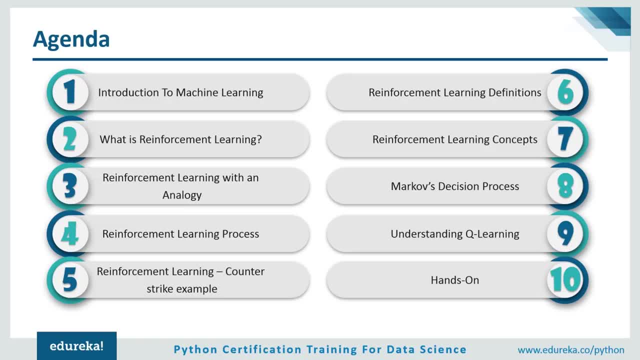 to first discuss the Q-learning algorithm with an example and we'll see how the Q-learning algorithm works. After that we'll move on to the hands-on part, where we'll be placing an agent in an unknown environment and he has to figure his way out of the environment. 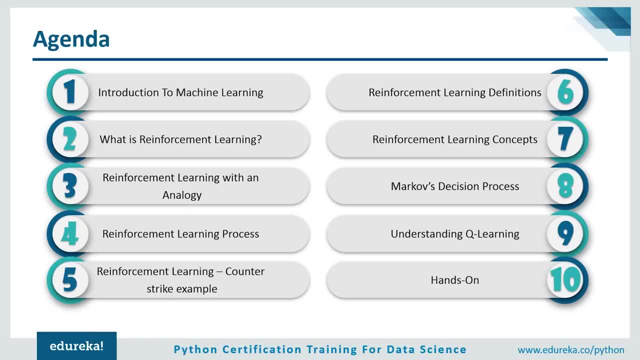 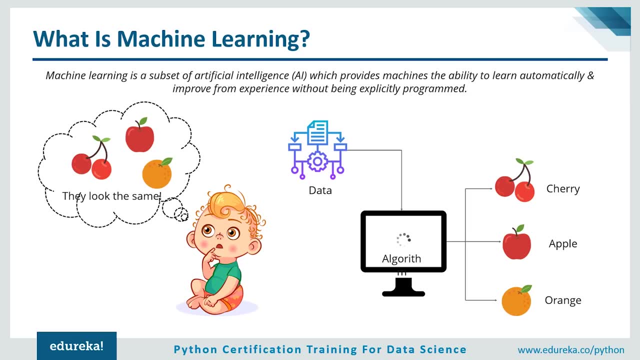 All right. so, guys, this is a very interesting demo, So let's start with our first topic, which is introduction to machine learning. So what is machine learning? Now, machine learning is the science of getting to know the machine. So machine learning is the science of getting 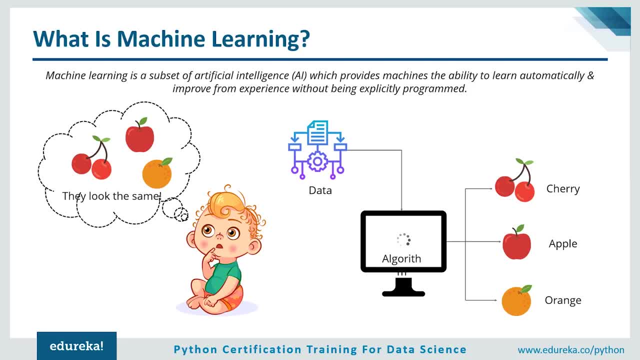 to know the machine. So machine learning is the science of getting to know the machine. Okay, so the machine is using computers to act, by feeding them data and letting them learn a few tricks on their own. Okay, so you're not actually programming the machine, but instead you're feeding. 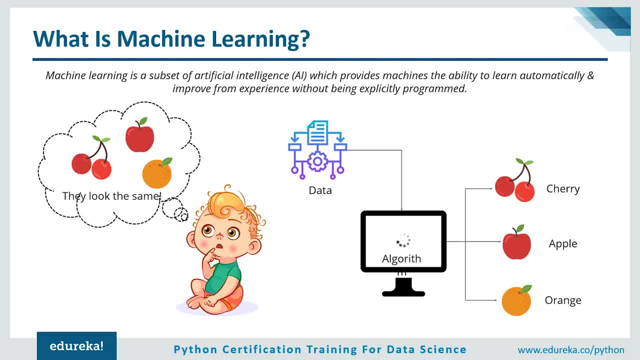 the machine a lot of data so that it can learn by itself. All right, so let's try to understand this with an example, So, as kids, we wouldn't be able to differentiate between the different fruits like apple, cherry and orange When we first see how apples, oranges and cherries look. we won't be. 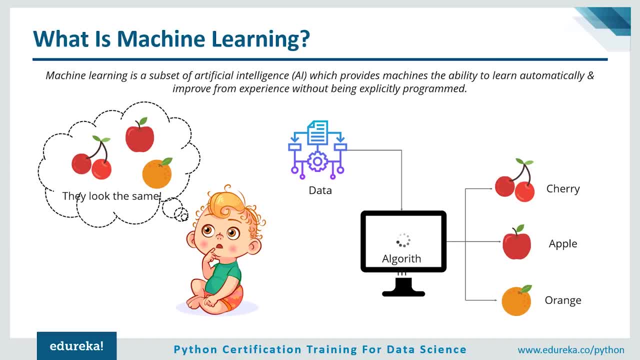 able to differentiate between them. This is because we haven't observed them enough. All right, we don't know how apples look, we don't know how cherries look and we don't know how oranges look, So we can't differentiate among them. But as we grow up and we learn how apples look, we know that. 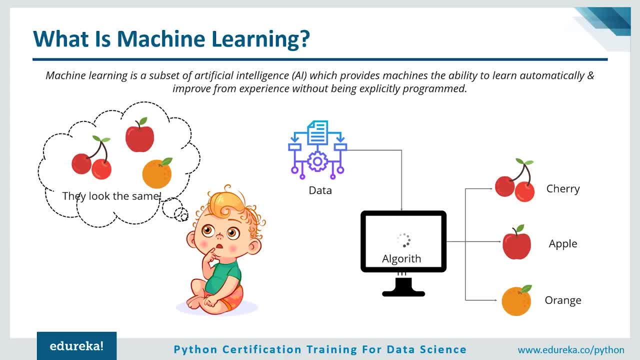 they're red in color and we know how cherries are smaller when compared to apples. we learn how to differentiate between the fruits. Similarly, when it comes to a machine, if you input images of an apple, orange and cherry to a machine, initially it won't be able to differentiate between the 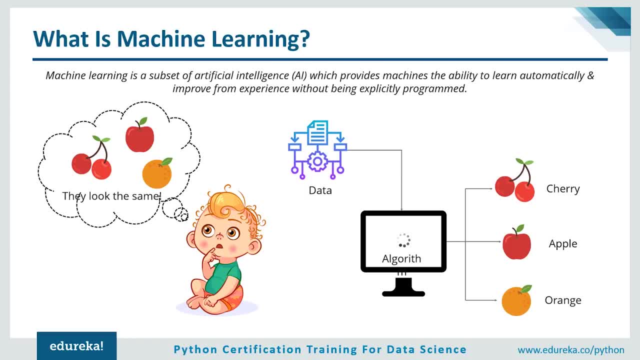 three. Now, this is because it doesn't have enough data about them. But if you keep feeding hundreds and thousands of images to the machine, it won't be able to differentiate between the three. So if you keep feeding hundreds and thousands of images to the machine about cherries, apples and 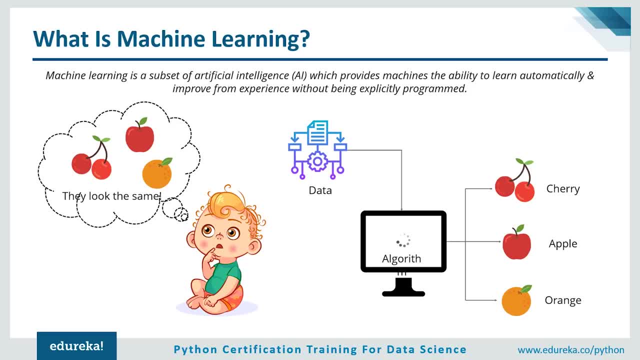 oranges, it'll learn how to differentiate between the three, Just like how we humans learn by looking around and observing and collecting data. Similarly, machines also learn when you give them a lot of data- All right. so when you input a lot of data to a machine, it'll learn how to. 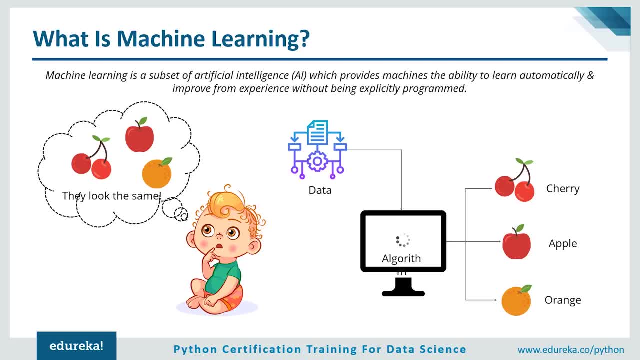 distinguish between them. So the machine will basically train on the data and it'll try to differentiate between the various fruits by using various machine learning algorithms. Now let's move ahead and look at how machines learn. There are three different types of machines that can. 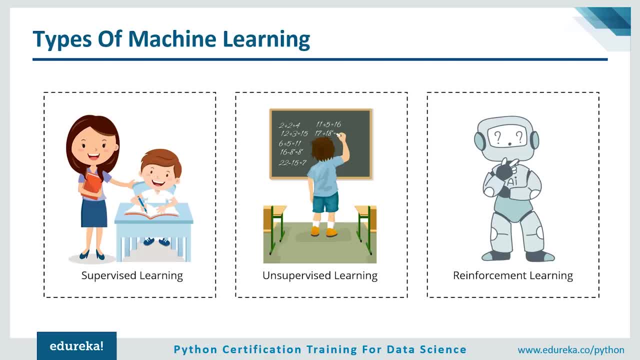 learn machine learning. Okay, so first we have the supervised learning. Now, supervised means to direct a certain activity and make sure it's done correctly. All right, So as children, when we attended school, we needed a lot of guidance from our teachers. All right, we couldn't solve a simple. 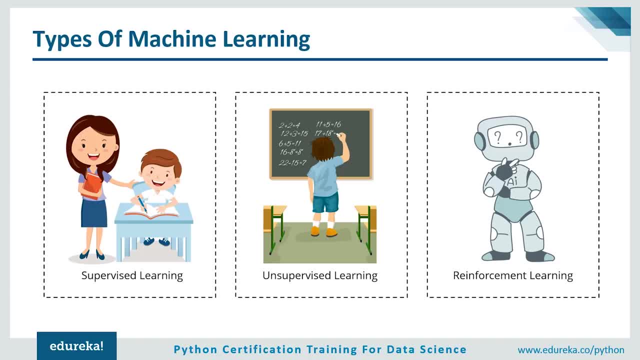 math problem if our teachers didn't practically show us how to do it. Okay, so we always needed a guide, which is basically the teacher, But later on we picked up our own pace. we learned how addition was done, how subtraction was done, All right, but initially we did. 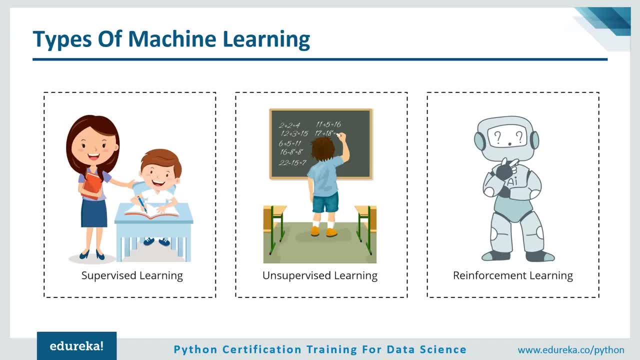 need a little bit of guidance. Now. this is exactly how supervised learning works. So if you feed the model a set of data called the training data, which contains both the input and the corresponding expected output, Okay so this training data will act like a teacher and it'll teach the model the 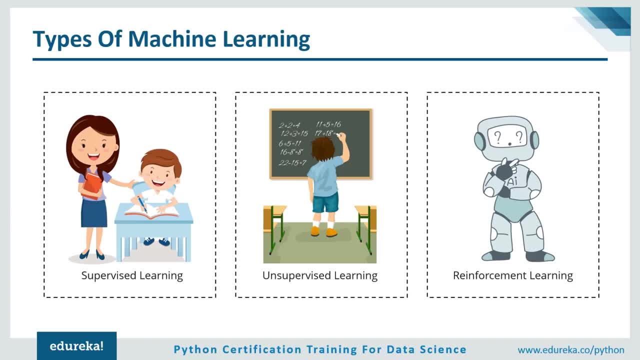 correct output for a particular input. So this was about supervised learning. Now, unsupervised means to act without anyone's direction or anyone's supervision. So, guys, when a child grows into an adult, we need to guide him at every step. Okay, so he observes and he learns without any help, And this 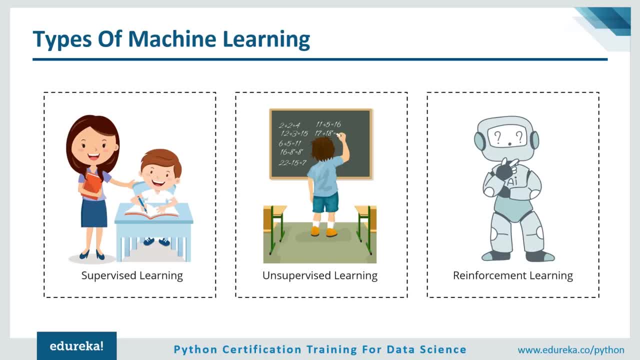 is exactly how unsupervised learning works. In this method, the model is basically given a data set which is neither labeled nor is it classified, So the machine doesn't know. okay, this is the input, so this is how the output should look, which means that if you input an image of a fruit, you're 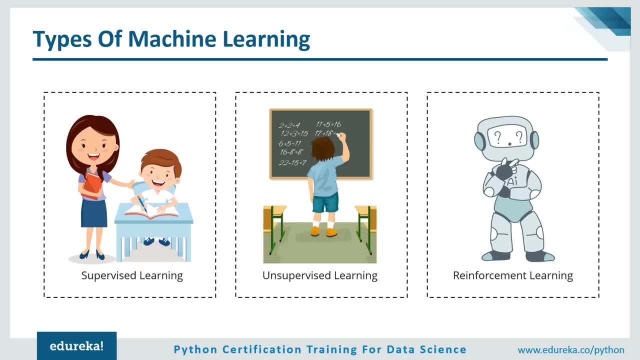 not going to label it as apple, Okay. instead, you're just going to give it data and the machine is going to learn on its own. All right, so next we have reinforcement learning. Now, reinforcement means to establish or encourage a pattern of behavior. So, guys, what would happen? 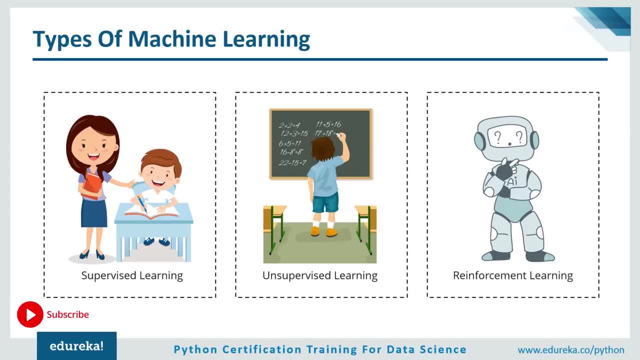 if you were dropped off, let's say, at an island- okay, at an isolated island. Initially you'd panic and be unsure of what to do, where to get food from, how to live and all of that. But after a while you have to adapt. you must learn how to live in the island, adapt to the changing climates. 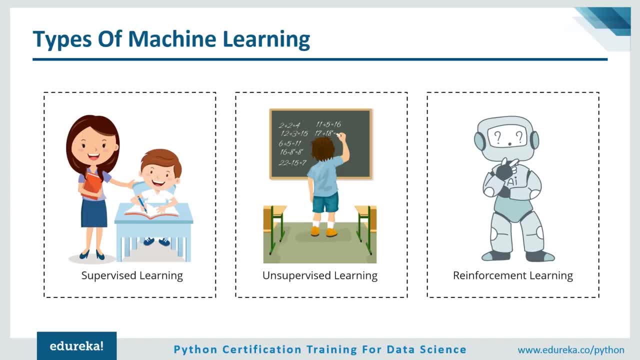 learn what to eat and what not to eat. Okay, so basically you're following the hit and trial concept, because you're new to the surrounding And the only way to learn is to experience and then learn from your experience. This is exactly what reinforcement. 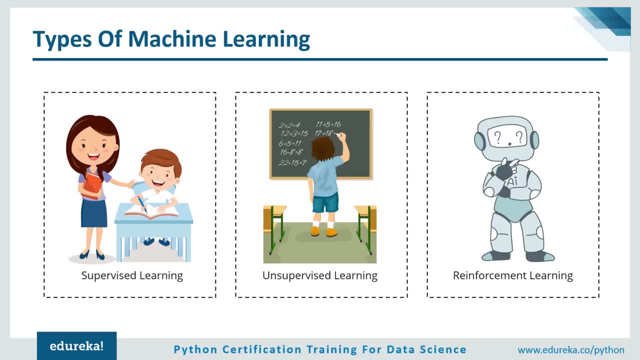 learning is? It is a learning method wherein an agent, which is basically you, stuck on the island, interacts with its environment, which is the island, by producing actions and discovering errors or rewards. Now, moving on, I'll be discussing more about reinforcement learning. 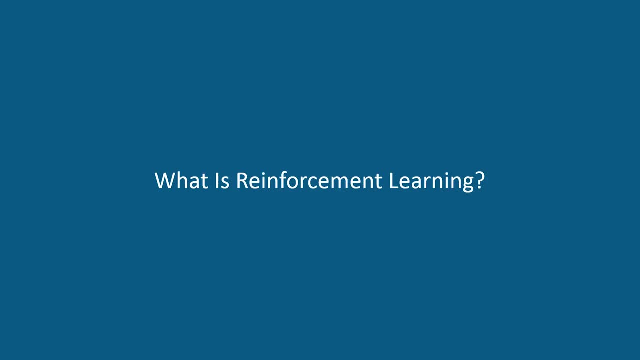 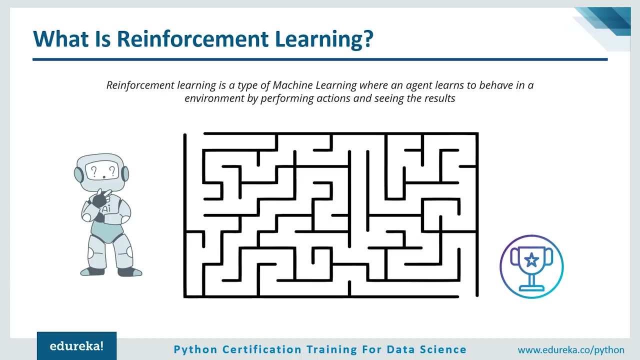 So let's look at some of the examples and let's define what reinforcement learning really is. So, guys, reinforcement learning is a part of machine learning, whereas reinforcement learning is a part of machine learning. So reinforcement learning is a. an agent is put in an environment and he learns to behave in this environment by performing. 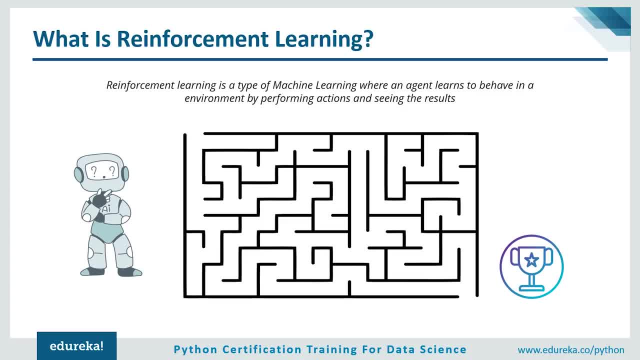 certain actions. Okay, so it basically performs actions and it either gets the rewards on the actions or it gets a punishment and observing the reward which it gets from those actions. Reinforcement learning is all about taking an appropriate action in order to maximize the 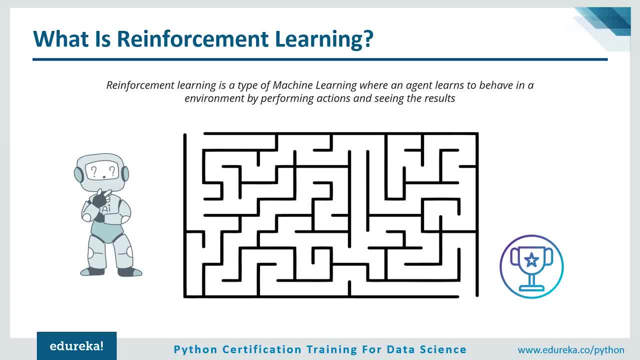 reward in a particular situation. So, guys, in supervised learning, the training data comprises of the input and the expected output, And so the model is trained with the expected output, And so the model is trained with the expected output. And so the model is trained with. 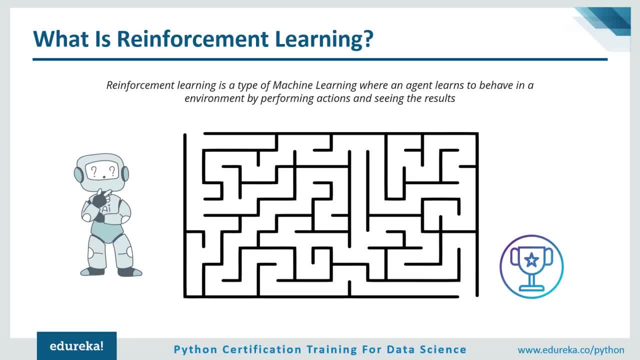 output itself. But when it comes to reinforcement learning, there is no expected output. Here, the reinforcement agent decides what actions to take in order to perform a given task. In the absence of a training data set, it is bound to learn from its experience itself. 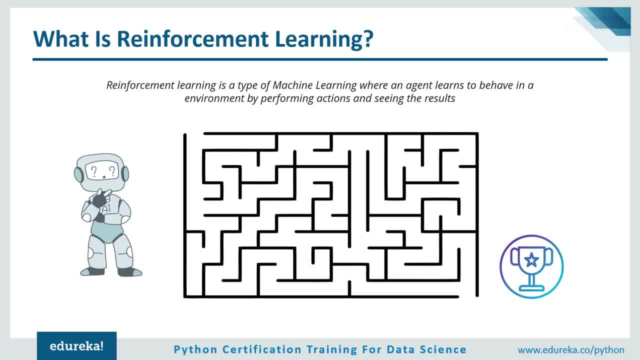 All right. So reinforcement learning is all about an agent who's put in an unknown environment and he's going to use a hit and trial method in order to figure out the environment and then come up with an outcome. Okay, now let's look at reinforcement learning with an analogy. 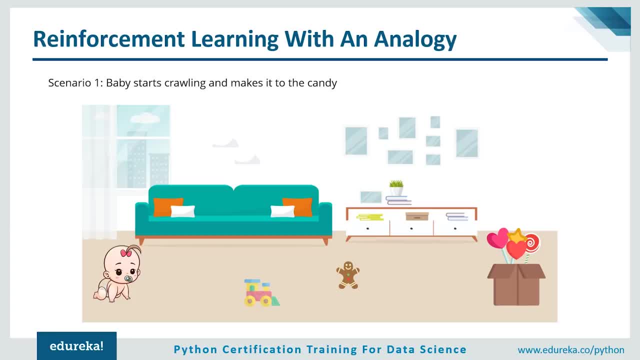 So consider a scenario wherein a baby is learning how to walk. This scenario can go about in two ways Now. in the first case, the baby starts walking and makes it to the candy. Here, the candy is basically the reward it's going to get. So since the candy is the end goal, the baby is happy. 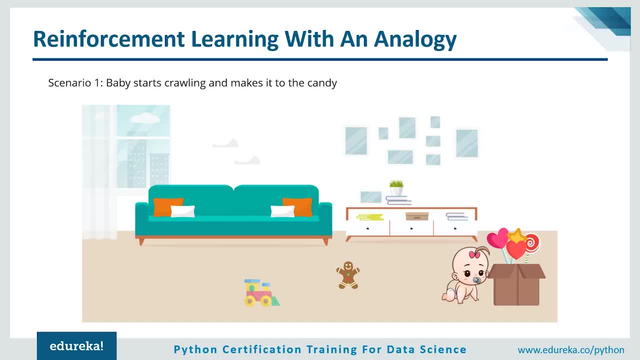 it's positive. Okay, so the baby is happy and it gets rewarded a set of candies. Now, another way in which this could go is that the baby starts walking but falls due to some hurdle in between. The baby gets hurt and it doesn't get. 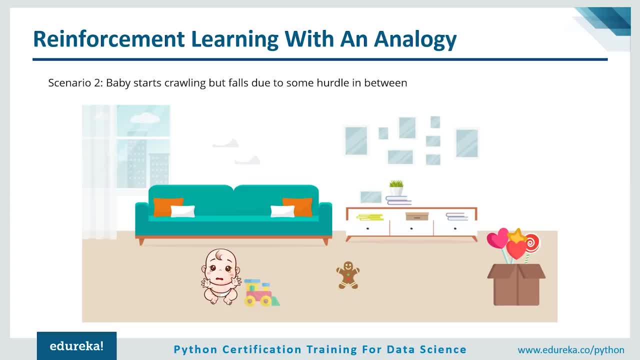 any candy And obviously the baby is sad. So this is a negative reward, Okay. or you can say this is a setback. So just like how we humans learn from our mistakes by trial and error, reinforcement learning is also similar, Okay, so we have an agent which is basically the baby. 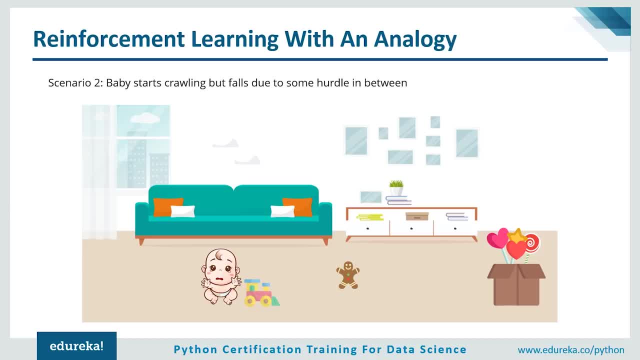 and a reward, which is the candy over here. Okay, And with many hurdles in between, the agent is supposed to find the best possible path to reach the reward. So, guys, I hope you all are clear with the reinforcement learning. Now let's look at the reinforcement learning process. 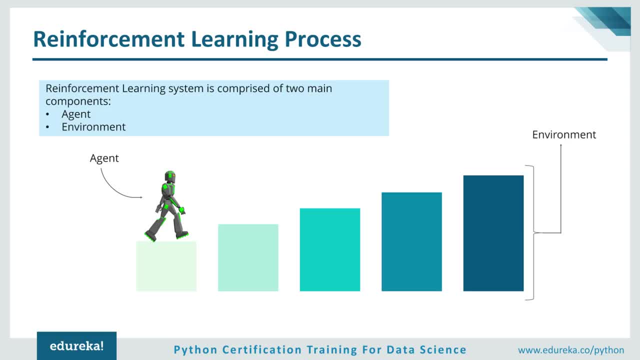 So, generally, a reinforcement learning system has two main components. All right, the first is an agent and the second one is an environment. Now, in the previous case we saw that the agent was a baby and the environment was a living room wherein the baby was crawling. Okay, the environment is. 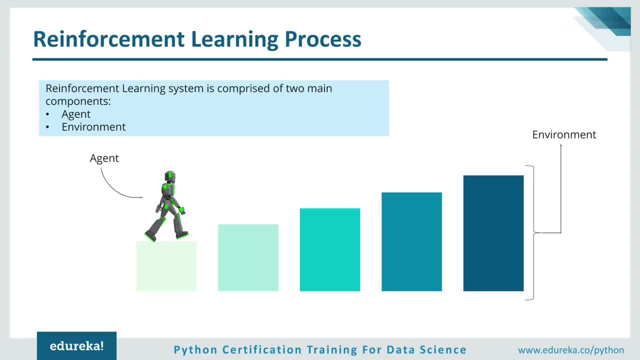 the setting that the agent is acting on. And the agent over here represents the reinforcement learning algorithm. So, guys, the reinforcement learning process starts when the environment sends a state to the agent, and then the agent will take some action. So the reinforcement learning, 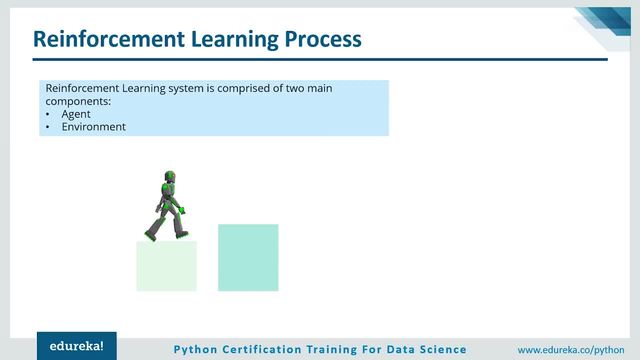 actions based on the observations. In turn, the environment will send the next state and the respective reward back to the agent. The agent will update its knowledge with a reward returned by the environment and it uses that to evaluate its previous action. So, guys, this loop keeps. 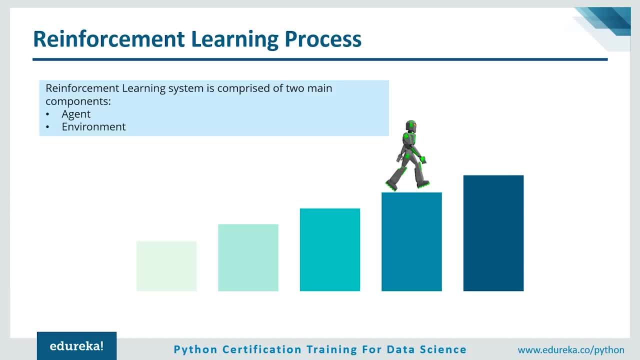 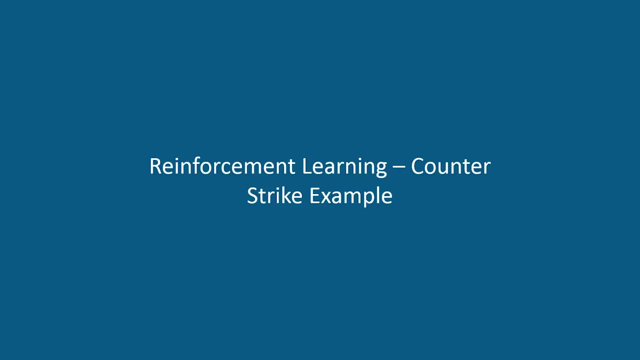 continuing until the environment sends a terminal state, which means that the agent has accomplished all his tasks and he finally gets the reward. Okay, this is exactly what was depicted in this scenario, So the agent keeps climbing up ladders until he reaches his reward. To understand this better, let's suppose that our agent is learning. 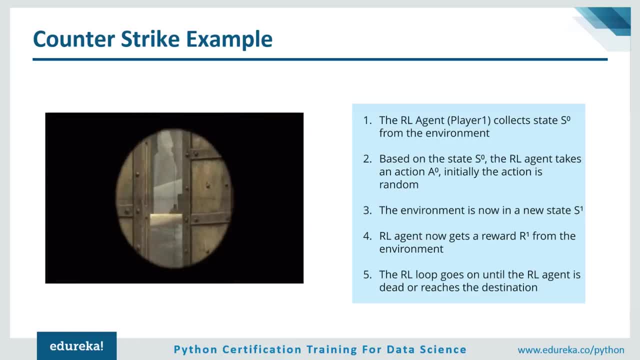 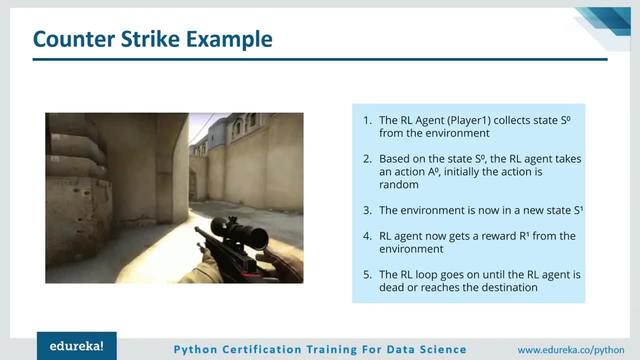 to play Counter-Strike. Okay, so let's break it down Now. initially, the RL agent, which is basically the player, player one, let's say it's the player one who is trying to learn how to play the game. Okay, he collects some state from the environment. Okay, this could be the first state. 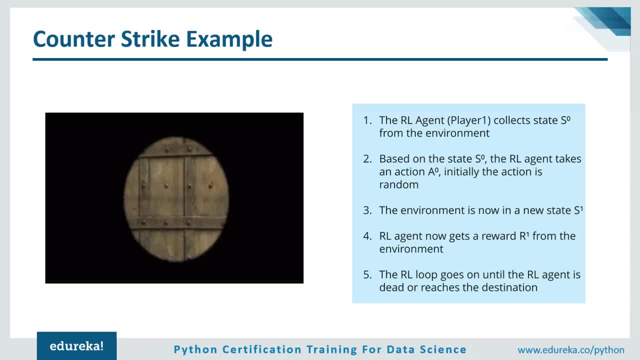 of Counter-Strike. Now, based on this state, the agent will take some action. Okay, and this action can be anything that causes a result. So if the player moves left or right, it's also considered as an action, Okay. so initially the action is going to be random because obviously 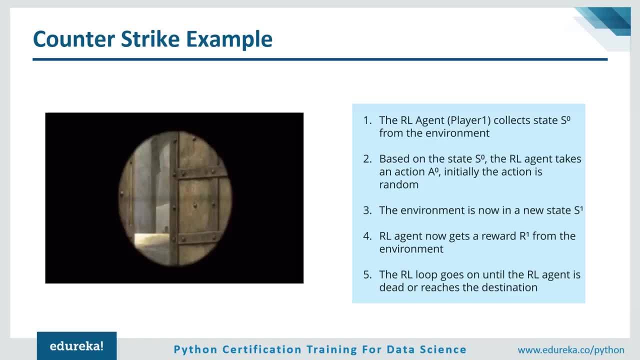 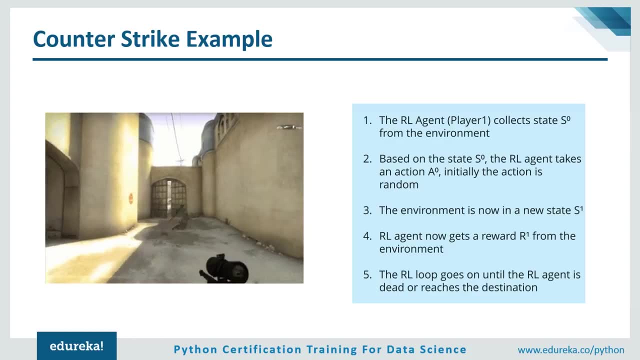 the first time you pick up Counter-Strike, you're not going to be a master at it, So you're going to try with different actions and you're just going to pick up a random action in the beginning. Now the environment is going to give a new state, So after clearing that, the environment is now 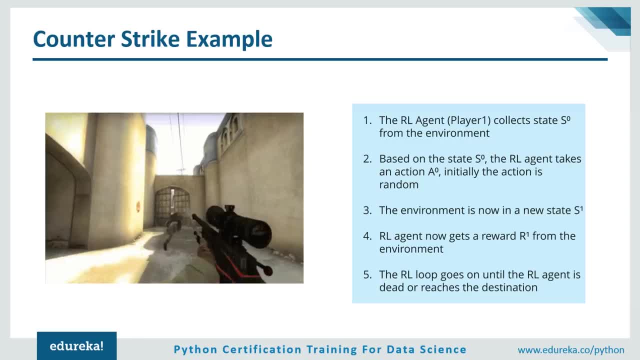 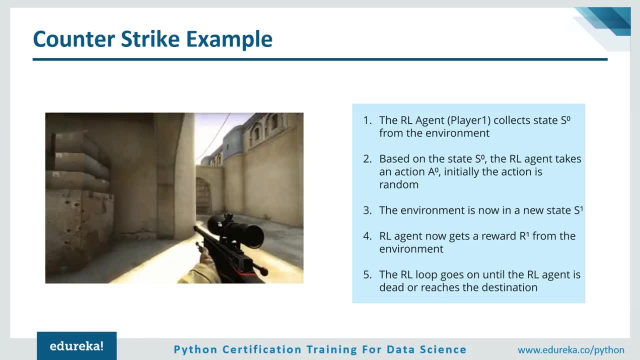 going to give a new state to the agent or to the player. So maybe he's crossed stage one. now he's in stage two. So now the player will get a reward- R1- from the environment because it cleared stage one. Reward can be anything. It can be additional points or coins or anything like that. Okay, so basically, 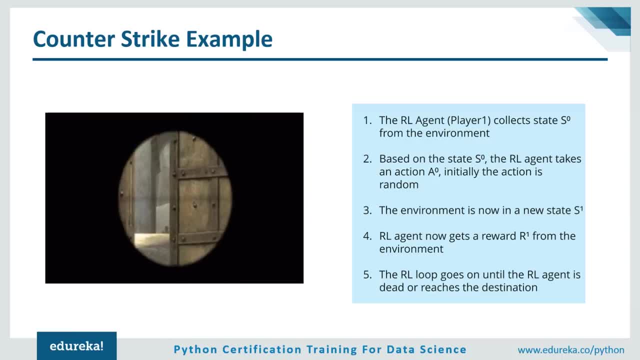 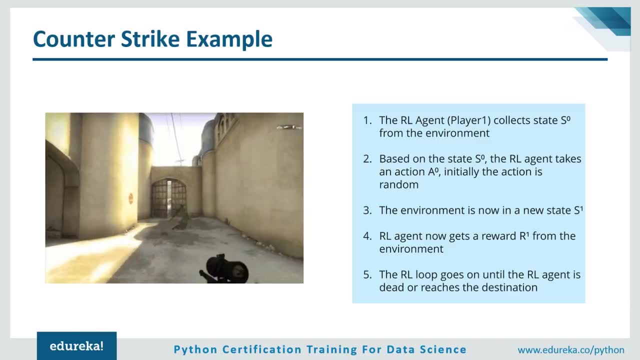 this loop keeps going on until the player is dead or reaches the destination Okay, and it continuously outputs a sequence of states, actions and rewards. So, guys, this was a small example to show you how reinforcement learning process works. So you start with an initial state and once the 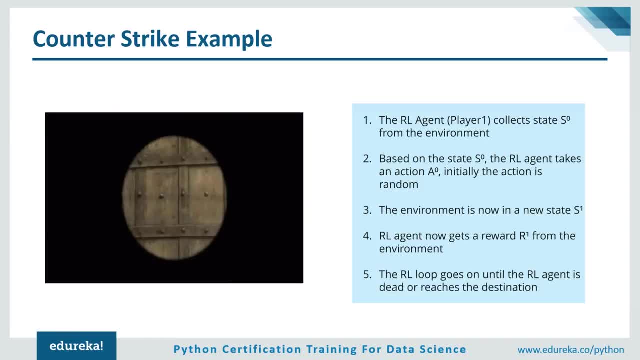 player clears that state, he gets a reward. After that, the environment will give another stage to the player and after it clears that state, it's going to get another reward. and it's going to keep happening until the player reaches his destination. All right, so, guys, I hope this is clear. Now let's move on and look at the 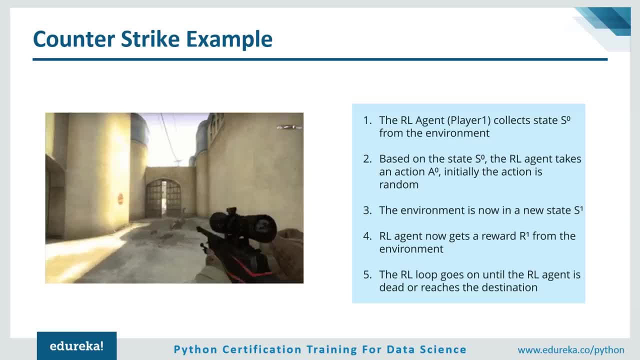 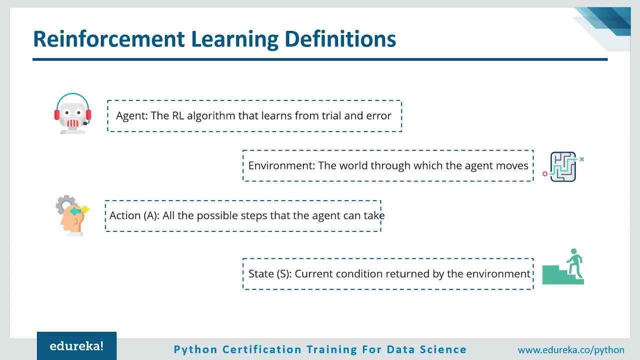 reinforcement learning definitions. So there are a few concepts that you should be aware of while studying reinforcement learning. Let's look at those definitions over here. So first we have the agent. Now an agent is basically the reinforcement learning algorithm that learns from trial and error. Okay, so an agent takes actions like, for example, a soldier encounters. 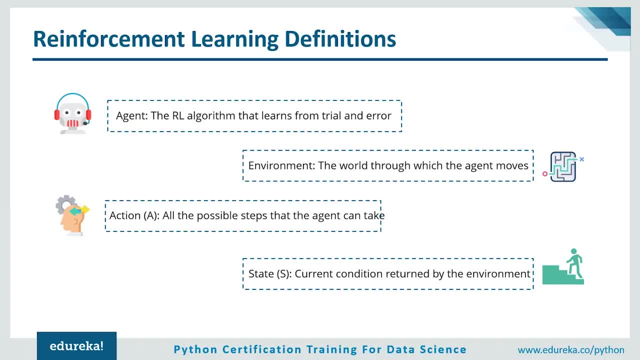 like navigating through the game, That's also an action. Okay, if he moves left, right or if he shoots at somebody, that's also an action. Okay. so the agent is responsible for taking actions in the environment. Now, the environment is the whole Counter-Strike game. Okay, it's basically the world. 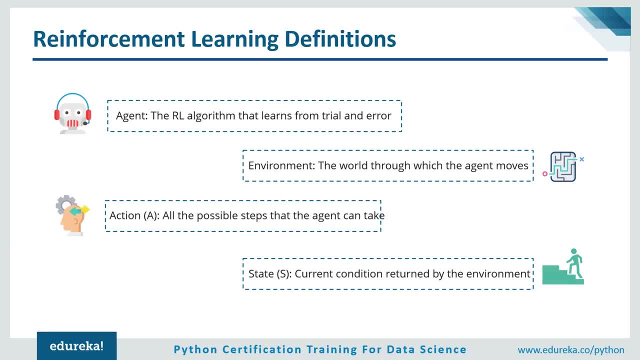 through which the agent moves The environment, takes the agent's current state and action as input and it returns the agent's reward and its next state as output. All right, next we have action. Now all the possible steps that an agent can take are: 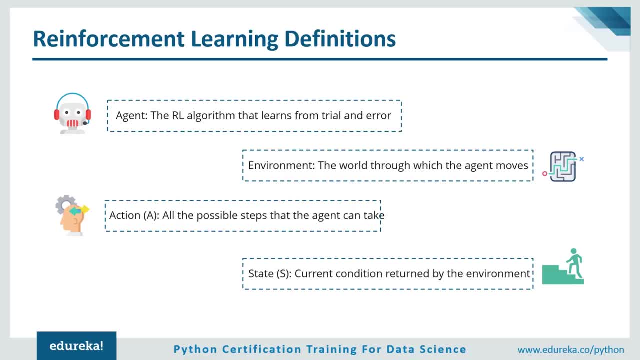 called actions. So, like I said, it can be moving right, left or shooting or any of that. All right, then we have state. Now, state is basically the current condition returned by the environment. So, whichever state you are in, if you're in state one or if you're in state two, that represents 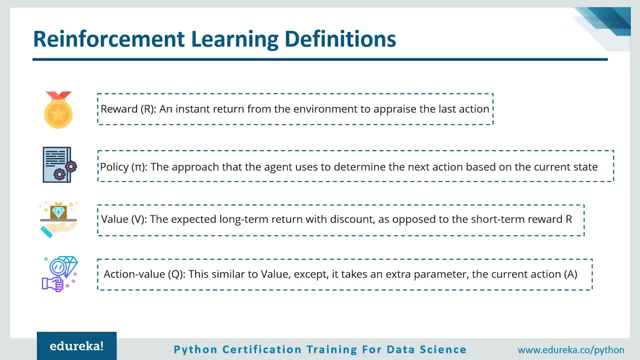 your current condition, All right. next we have reward. A reward is basically an instant return from the environment to appraise your last action. Okay, so it can be anything like coins or it can be additional points. So basically, a reward is an instant return from the environment to appraise. 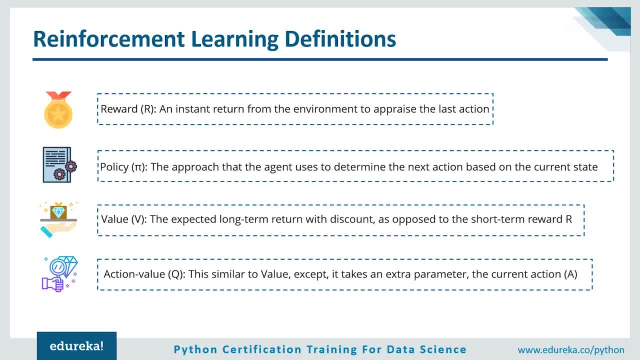 what is given to an agent after it clears the specific stages. Next we have policy. Policy is basically the strategy that the agent uses to find out his next action based on his current state. Policy is just the strategy with which you approach the game. Then we have value. Now, value is the. 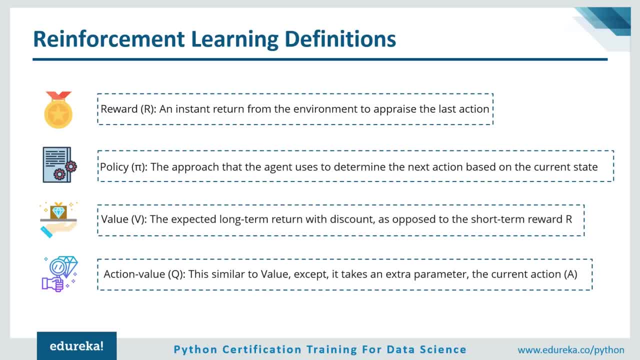 expected long-term return with discount. So value and action value can be a little bit confusing for you right now, But as we move further you'll understand what I'm talking about. Okay, so value is the long-term return that you get with discount. Okay, discount, I'll explain in the further. 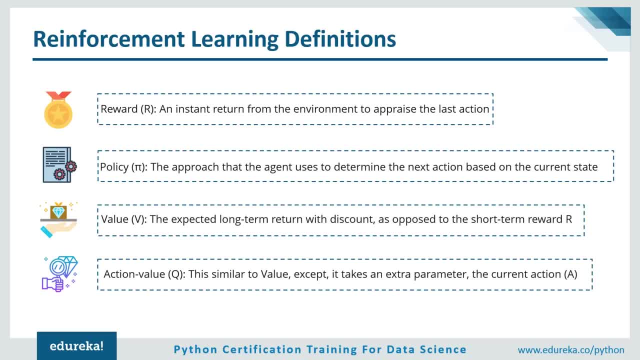 slides. Then we have action value. Now action value is also known as Q value. Okay, it's very similar to value, except that it takes an extra parameter, which is the current action. So, basically, here you'll find out the Q value, depending on the particular action that you took. 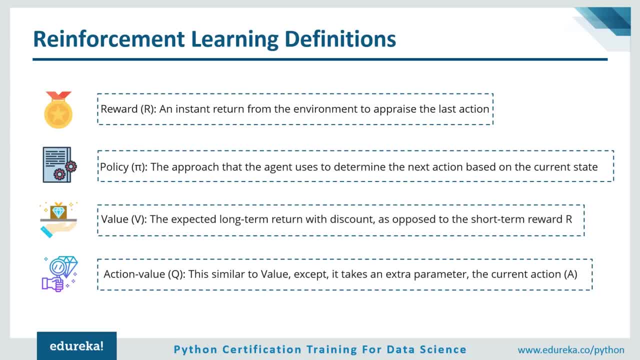 All right. so, guys, don't get confused with value and action value. We look at examples in the further slides and you'll understand this better. Okay, so, guys, make sure that you're familiar with terms, because you'll be seeing a lot of these terms in the further slides. All right Now before. 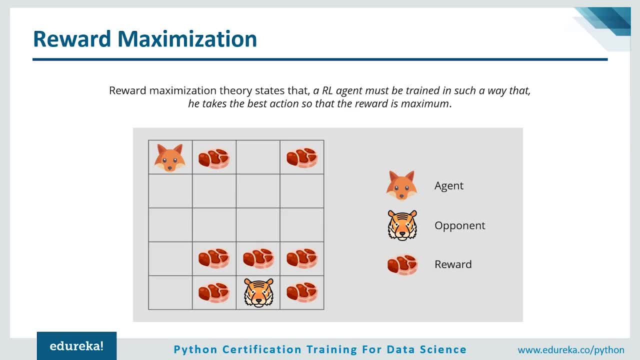 we move any further, I'd like to discuss a few more concepts. Okay, so first we'll discuss the reward maximization. So, if you haven't already realized it, the basic aim of the RL agent is to maximize the reward. Now, how does that happen? Let's try to understand this in depth. So the agent must be. 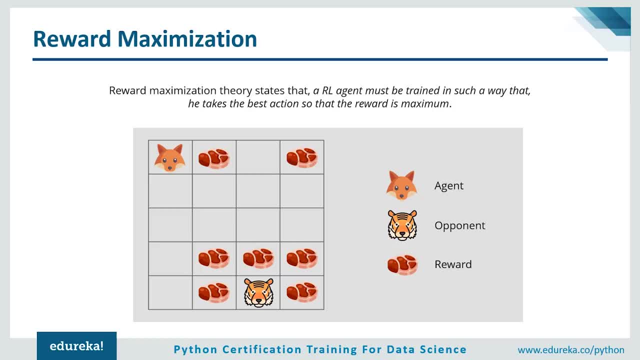 trained in such a way that he takes the best action so that the reward is maximum, because the end goal of reinforcement is to maximize the reward. So the end goal of reinforcement is to maximize the reward. So the end goal in learning is to maximize your reward based on a set of actions. So let me explain this with a 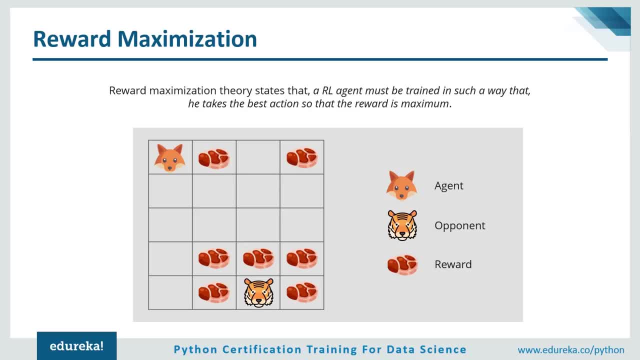 small game. Now in the figure you can see there is a fox, there's some meat and there's a tiger. So our agent is basically the fox, and his end goal is to eat the maximum amount of meat before being eaten by the tiger. Now, since the fox is a clever fellow, he eats the meat that is closer to. 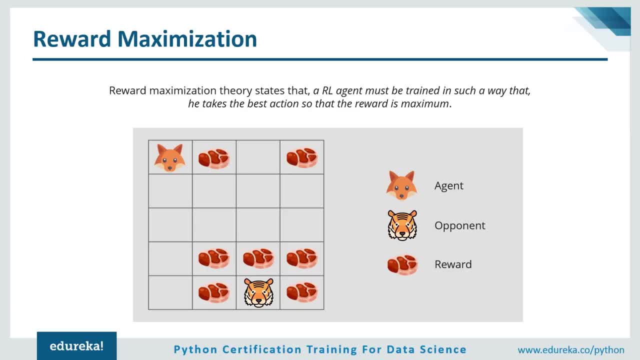 him rather than the meat, which is closer to the tiger. Now, this is because the closer he is to the tiger, the higher are his chances of getting killed. So because of this, the agent must be trained in such a way that he can eat the maximum amount of meat before being eaten by the tiger. So 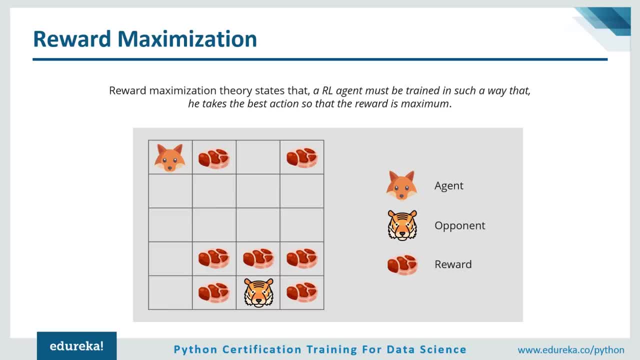 because of this, the rewards which are near the tiger, even if they are bigger meat chunks, they will be discounted. So this is exactly what discounting means. So our agent is not going to eat the meat chunks which are closer to the tiger because of the risk. Now, even though the meat 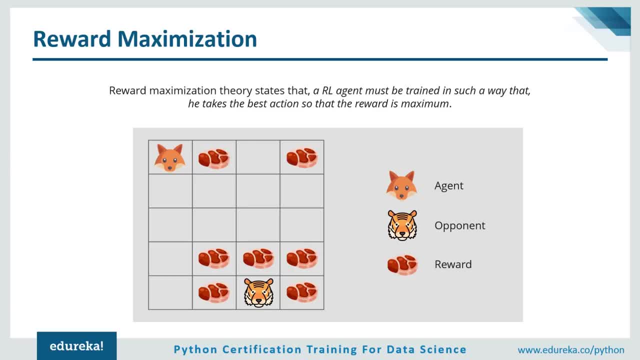 chunks might be larger. he does not want to take the chances of getting killed. This is called discounting. This is where you discount, because you improvise and you just eat the meat which are closer to you, instead of taking risks and eating the meat which are closer to your opponent Now. 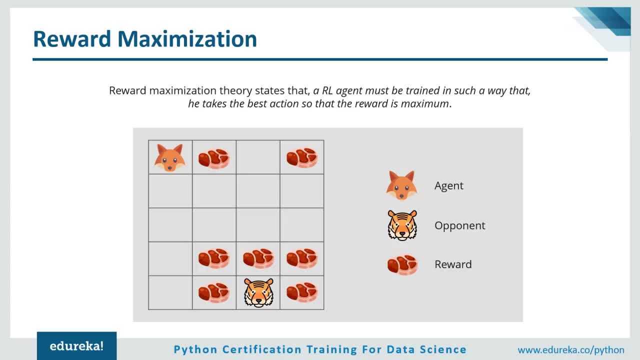 the discounting of reward works based on a value called gamma. We'll be discussing gamma in our further slides, But, in short, the value of gamma is between zero and one. Okay, so the smaller the gamma, the larger is the discount value. Okay, so if the gamma value is lesser, it means that the 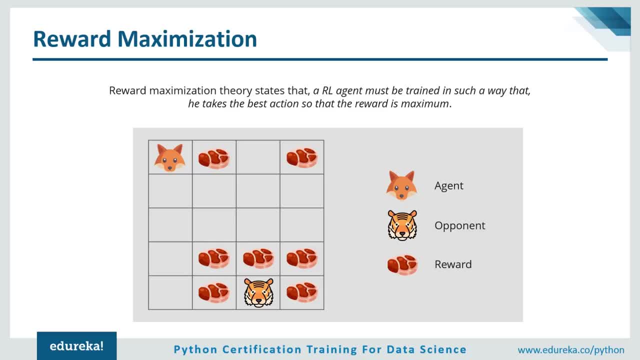 agent is not going to explore and he's not going to try and eat the meat chunks which are closer to the tiger. Okay. but if the gamma value is closer to one, it means that our agent is actually going to explore and it's going to try and eat the meat chunks which are closer to the tiger, Okay. 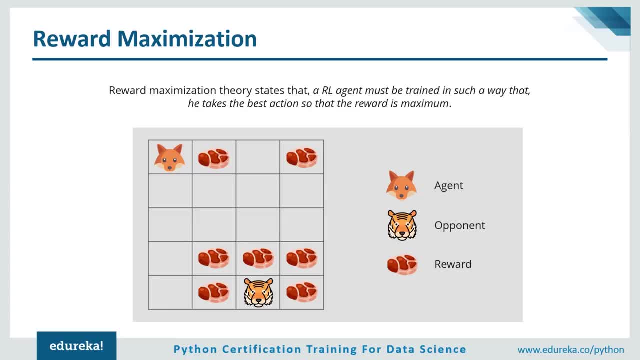 the meat chunks which are closer to the tiger. All right Now. I'll be explaining this in depth in the further slides, So don't worry if you haven't got a clear concept yet, but just understand that reward maximization is a very important step when it comes to reinforcement learning, because the 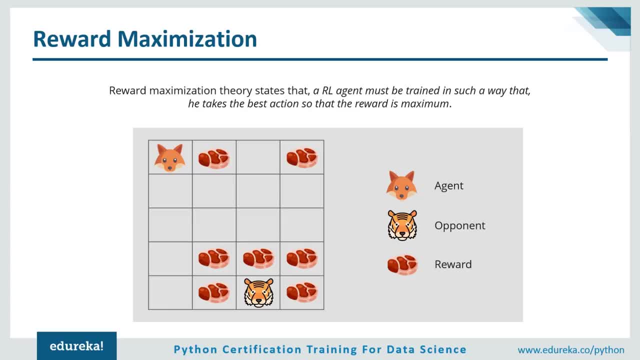 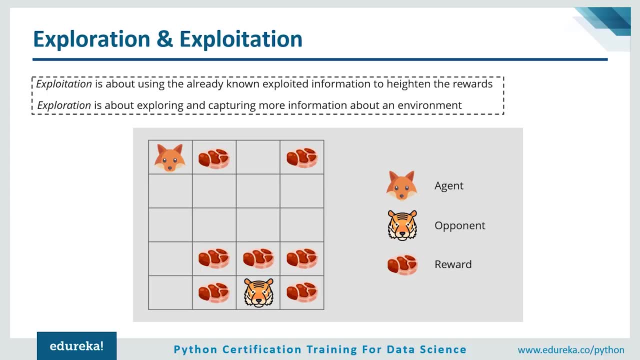 agent has to collect maximum rewards by the end of the game. All right, Now let's look at another concept, which is called exploration and exploitation. So exploration, like the name suggests, is about exploring and capturing more information about an environment. On the other hand, exploitation is about using the already known, exploited information. 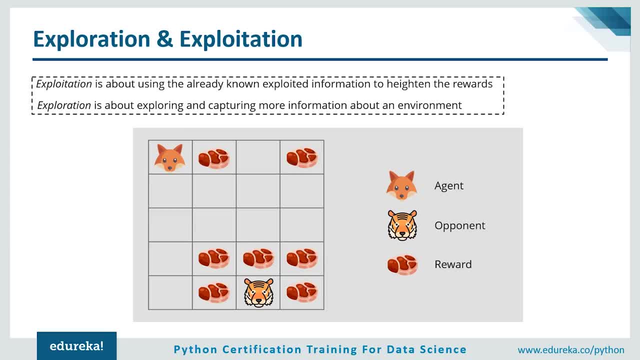 to heighten the rewards. So guys consider the fox and tiger example that we discussed Now here. the fox eats only the meat chunks which are close to him, but he does not eat the meat chunks which are closer to the tiger. Okay, even though they might give him more rewards, he does. 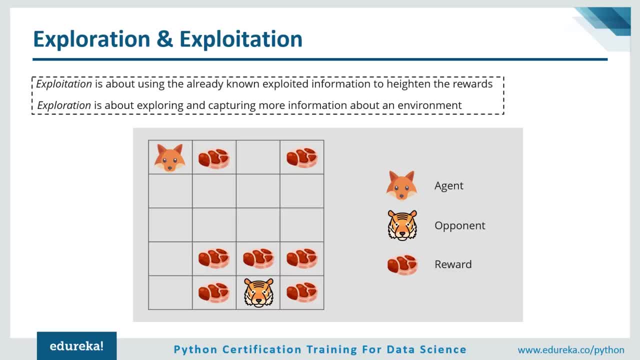 not eat them. If the fox only focuses on the closest rewards, he will never reach the big chunks of meat. Okay, this is what exploitation is about. You're just going to use the currently known information and you're going to try and get rewards based on that information. But if the 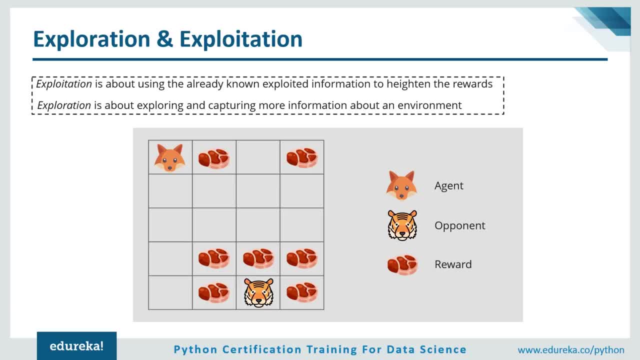 fox decides to explore a bit, it can find the bigger reward, which is the big chunks of meat. This is exactly what exploration is. So the agent is not going to stick to one corner. Instead, he's going to explore the entire environment and try and collect bigger rewards. All right, So, guys. 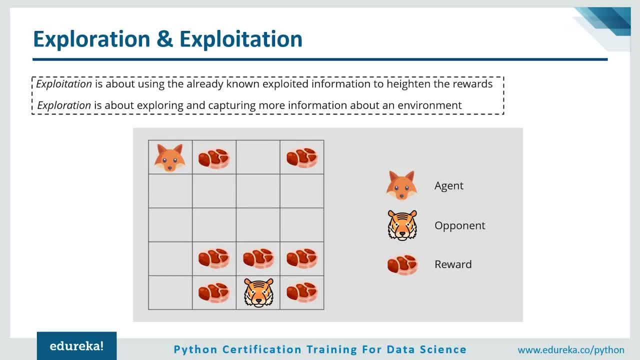 I hope you all are clear with exploration and exploitation. Now let's look at the Markov's decision process. So, guys, this is basically a mathematical process. So let's look at the Markov's decision process. So, guys, this is basically a mathematical process. So, guys, this is. 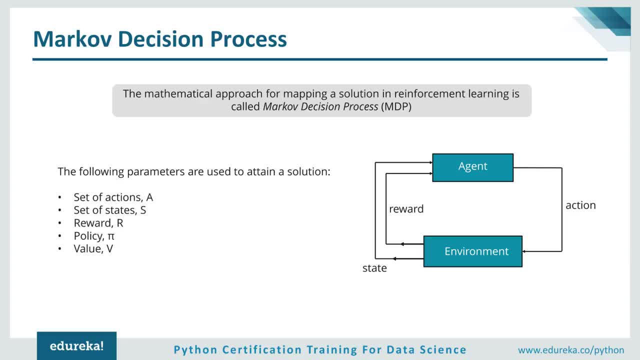 a mathematical approach for mapping a solution in reinforcement learning. In a way, the purpose of reinforcement learning is to solve a Markov decision process. Okay, so there are a few parameters that are used to get to the solution. So the parameters include the set of actions, the set of states, 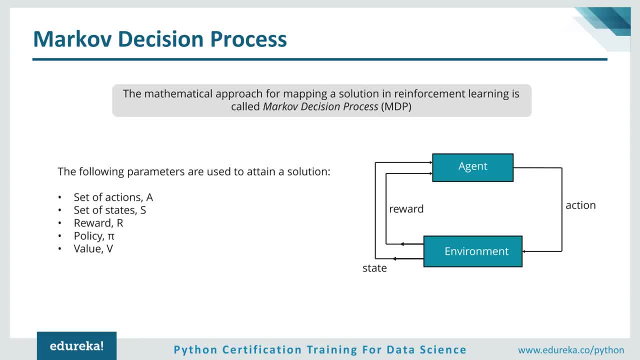 the rewards, the policy that you're taking to approach the problem and the value that you get. Okay, so, to sum it up, the agent must take an action A to transition from a start state to the end state S. While doing so, the agent will receive a reward R for each action that he takes. So, guys, a series. 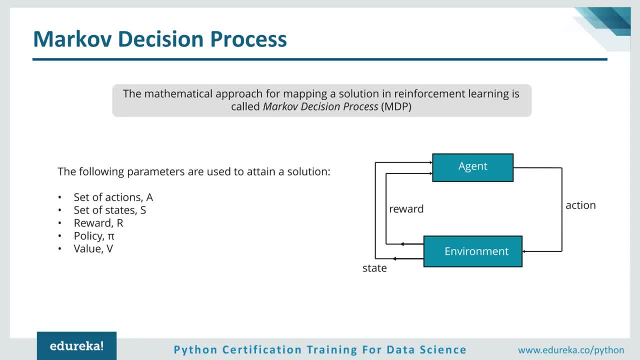 of actions taken by the agent define the policy, or it defines the approach, And the rewards that are collected define the value. So the main goal here is to maximize the rewards by choosing the optimum policy. All right, Now let's try to understand this with the help of the shortest path problem. 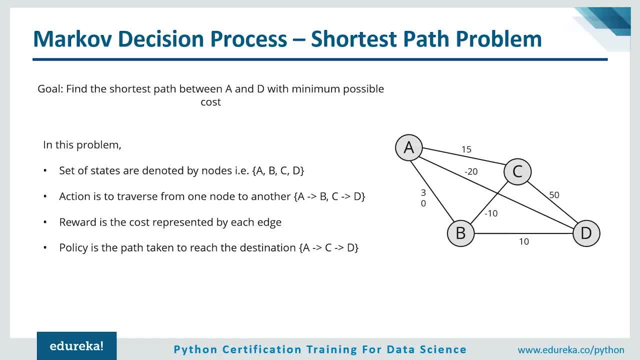 I'm sure a lot of you might have gone through this problem when you were in college. So, guys, look at the graph over here. So this is the shortest path problem. And this is the shortest path problem. So our aim here is to find the shortest path between A and D with minimum possible cost. So the value: 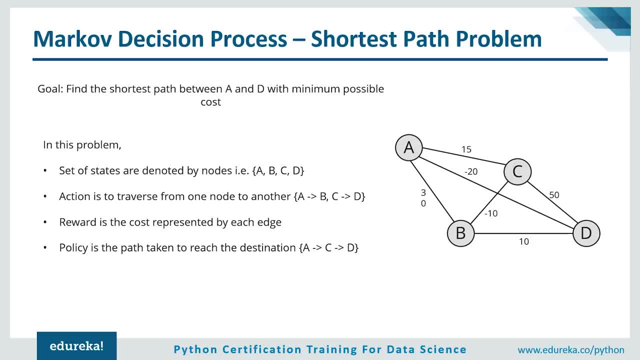 that you see on each of these edges basically denotes the cost. So if I want to go from A to C, it's going to cost me 15 points. Okay, so let's look at how this is done Now before we move, and 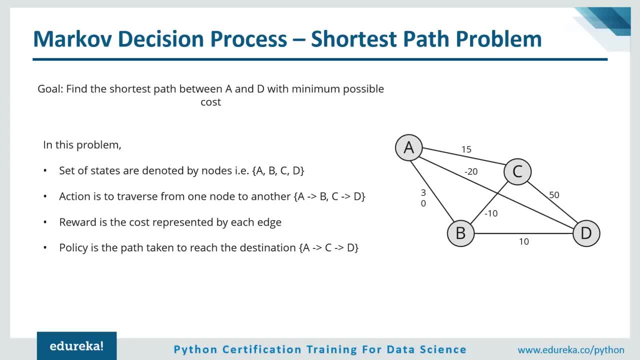 look at the problem. in this problem, the set of states are denoted by the nodes, which is A, B, C, D, And the action is to traverse from one node to the other. So if I'm going from A to B, that's an. 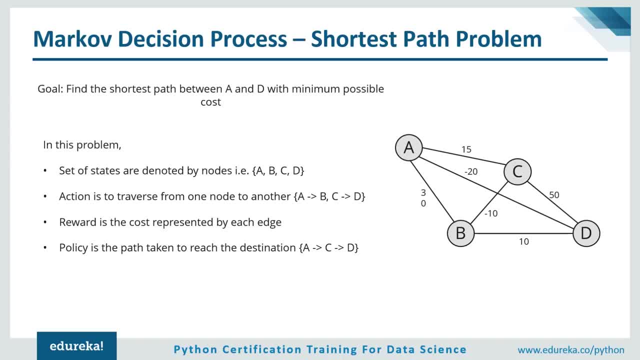 action. Similarly A to C, that's an action. Okay. the reward is basically the cost, which is represented by each edge over here. All right, Now the policy is basically the path that I choose to reach the destination. So let's say I choose A, C, D. Okay, that's one policy. In order to get to D, I'm. 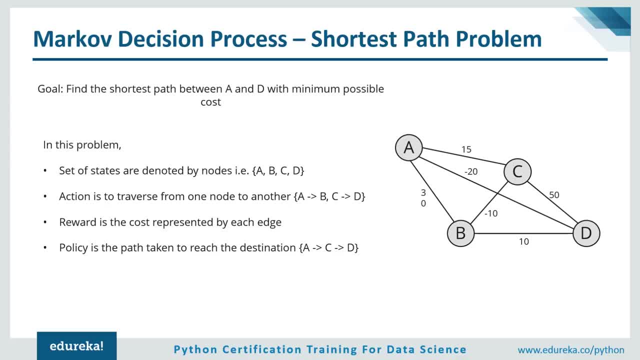 choosing A, C, D, which is a policy. Okay, it's basically how I'm approaching the problem. So, guys, here you can start off at node A and you can take baby steps to your destination. Now, initially you're clueless, So you can just take. 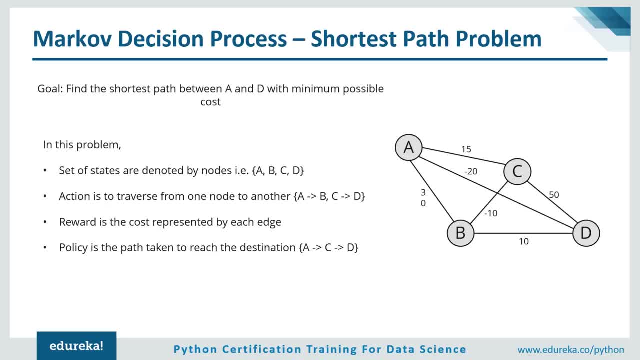 the next possible node which is visible to you. So, guys, if you're smart enough, you're going to choose A to C instead of A B C D or A B D. All right, So now, if you're at node C, you want. 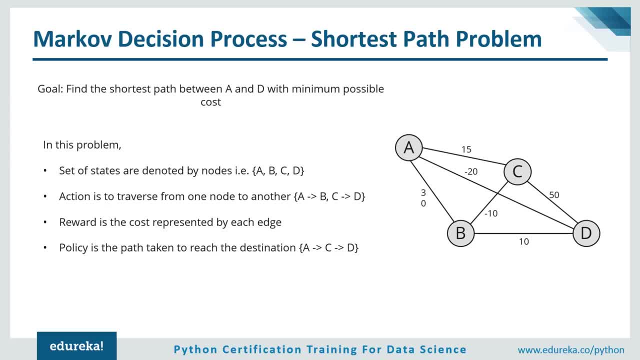 to traverse to node D, You must again choose a wise path. All right, You just have to calculate which path has the highest cost or which path will give you the maximum rewards. So, guys, this is a simple problem. We're just trying to calculate the shortest path between A and D by traversing 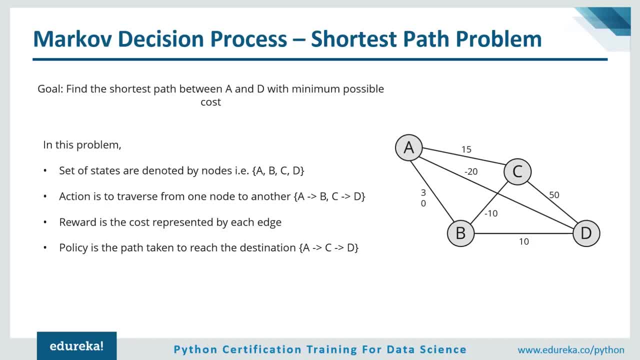 through these nodes. So if I traverse from A to C, which is the shortest path between A and D, it gives me the maximum reward. Okay, It gives me 65, which is more than any other policy would give me. Okay. So if I go from A, B, D, it would be 40. When you compare this to A, C, D, it gives. 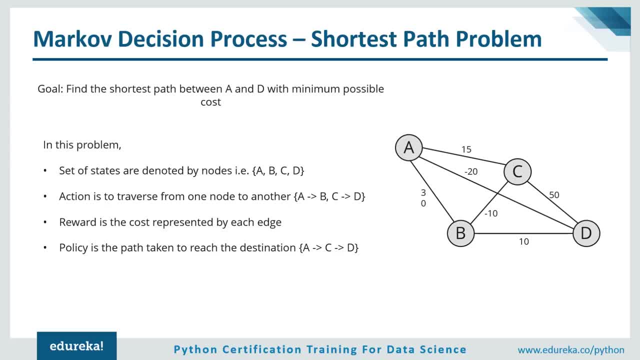 me more rewards. So obviously I'm going to go with A, C, D, Okay. So, guys, it was a simple problem, in order to understand how Markov decision process works, All right. So, guys, I want to ask you a. 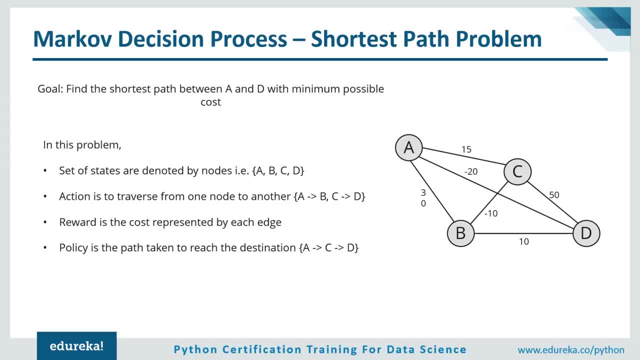 question: What do you think I did here? Did I perform exploration or did I perform exploitation? Now, the policy for the example is of exploitation, because we didn't explore the other nodes. Okay, We just selected three nodes and we traverse through them. So that's why this is called exploitation. We must 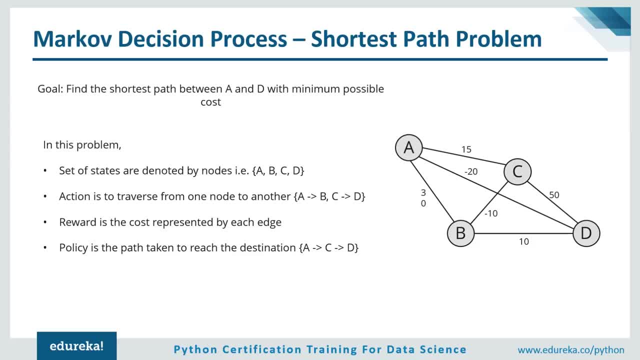 always explore the different nodes so that we can find a more optimal policy. But in this case obviously A C D has the highest reward and we're going with A C D. But generally it's not so simple. There are a lot of nodes, There are hundreds of nodes to traverse and there are, like 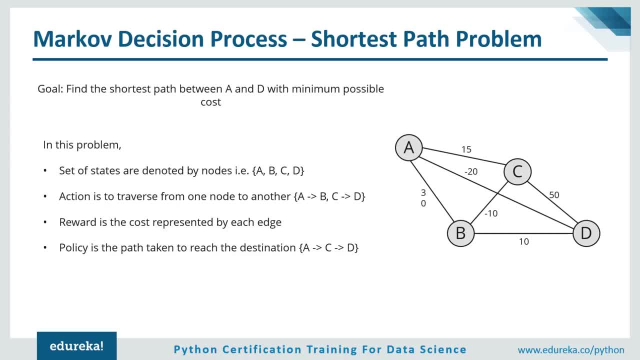 50, 60 policies. Okay, 50, 60 different policies. So you make sure you explore through all the policies and then you explore the other nodes. So that's why this is called exploitation, Okay. So, guys, before we perform the hands-on part, let's try to understand the math behind our 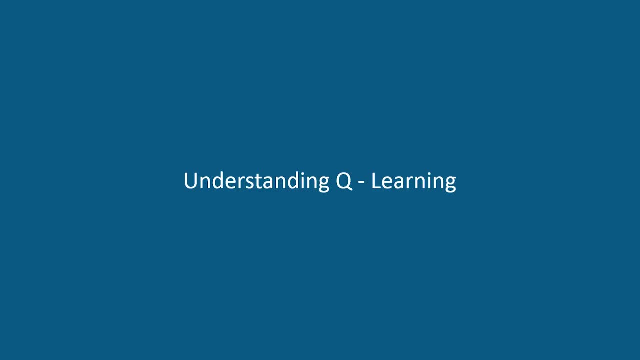 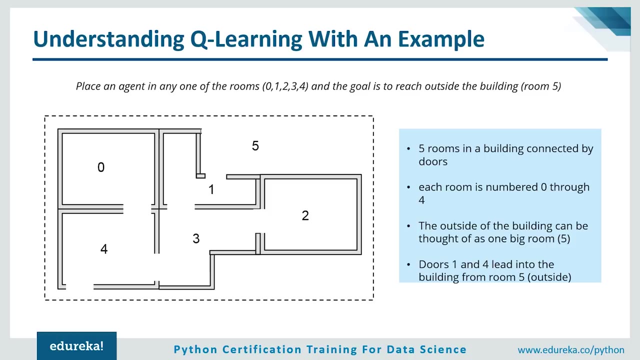 demo. Okay, So in our demo, we'll be using the Q learning algorithm, which is a type of reinforcement learning algorithm. Okay, It's simple. It just means that you have to take the best possible actions to reach your goal or to get the most rewards. All right, Let's try to. 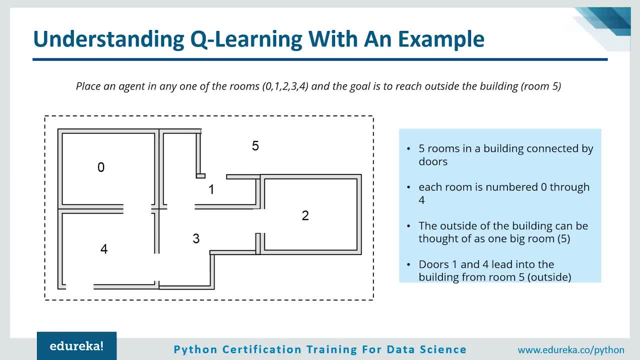 understand this with an example. So, guys, this is exactly what will be running in our demo, So make sure you understand this properly. Okay, So our goal here is we're going to place an agent in any one of the rooms. Okay, So, basically, these squares, you see, here are rooms. Okay, Zero is a room Four. 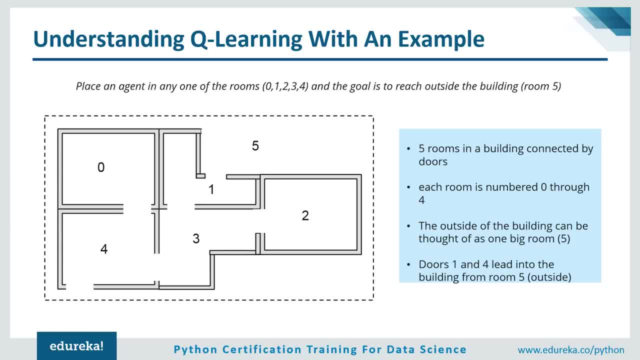 is a room, Three is a room, One is a room and two is a room, Five is also a room. It's basically a way outside the building, All right. So what we're going to do is we're going to place an agent in. 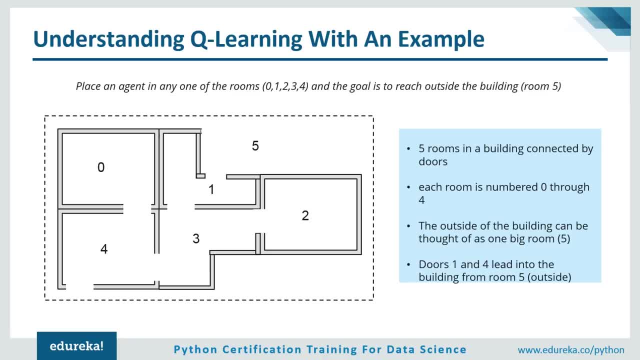 any one of these rooms And the goal is to reach outside the building. Okay, Outside the building is room number five. Okay, So these empty spaces are basically doors, which means that you can go from zero to four, You can go from four to three, three to one. 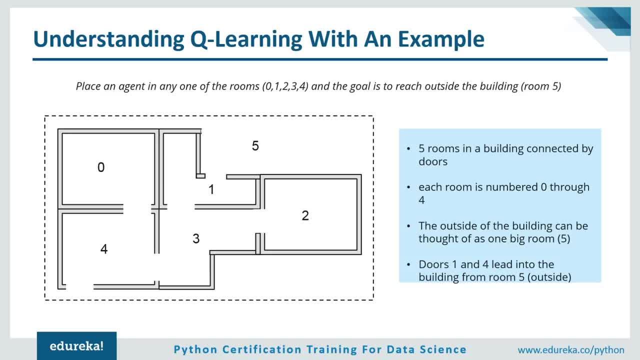 one to five and similarly three to two, But you can't go from five to two directly, All right, So there are certain set of rooms that don't get connected directly. Okay, So, like I've mentioned here, each room is numbered from zero to four and the outside of the building is numbered as five. 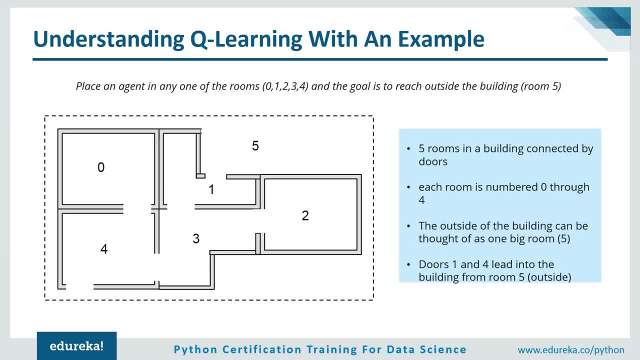 And one thing to note here is: room one and room four directly lead to room number five. All right, So room number one and four Will directly lead out to room number five. So basically our goal over here is to get to room number five. Okay, To set this room as a goal, we'll associate a reward value to each door. 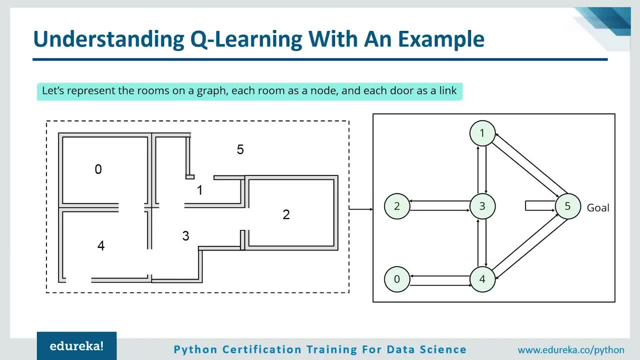 Okay, Don't worry, I'll explain what I'm saying. So, if you represent these rooms in a graph, this is how the graph is going to look. Okay, So, for example, from two you can go to three and then three to one, one to five, which will lead us to our goal. These arrows represent the 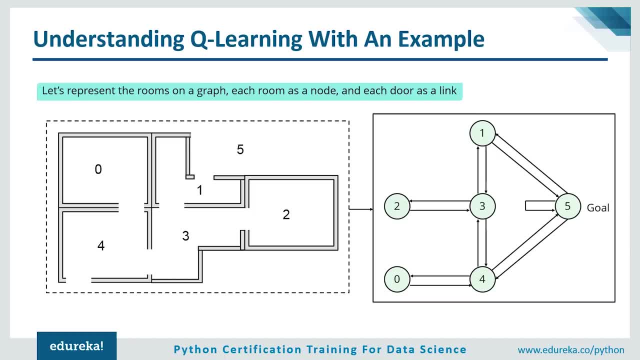 link between the doors. All right, This is quite understandable. All right, So let's go to room four. This is quite understandable. Now our next step is to associate a reward value to each of these doors. Okay, So the rooms that are directly connected to our end room, which is room number. 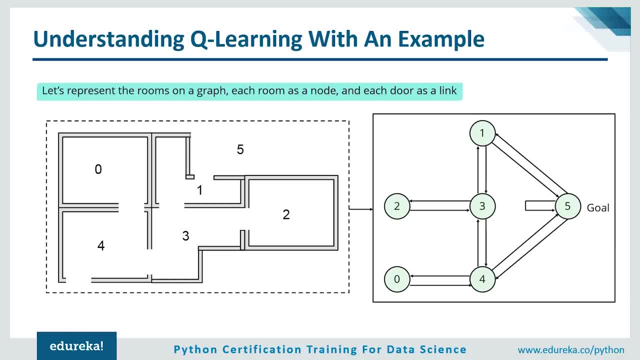 five, we'll get a reward of a hundred. Okay, So, basically, our room number one will have a reward five. Now, this is obviously because it's directly connected to five. Similarly, four will also be associated with a reward of a hundred because it's directly connected to five. Okay, So, if you go out, 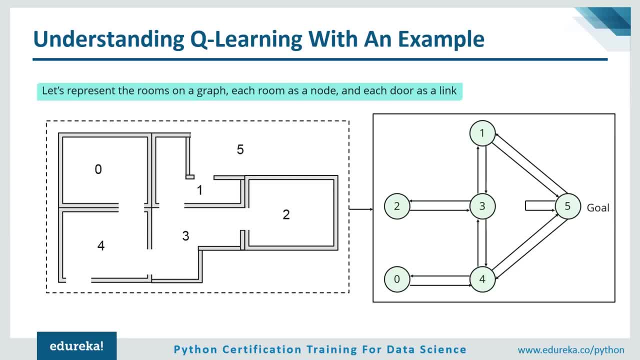 from four, it'll lead to five. Now, the other nodes are not directly connected to five. So if you go out from four, it'll lead to five. Now, the other nodes are not directly connected to five. So if you go out from four, it'll lead to five. Now, the other nodes are not directly connected to five. So if you go 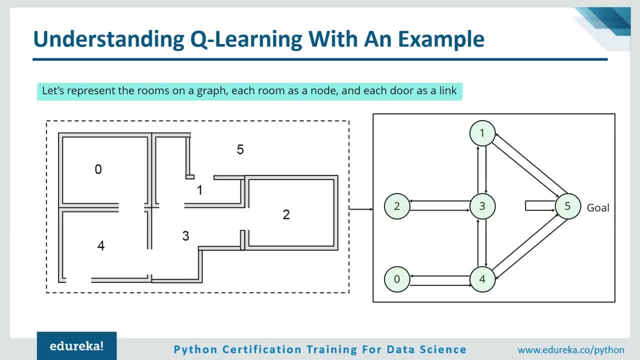 can't directly go from zero to five. Okay, So for this we'll be assigning a reward of zero. So, basically, other doors not directly connected to the target room have a zero reward. Okay Now, because the doors are two way, the two arrows are assigned to each room. Okay, You can see two arrows. 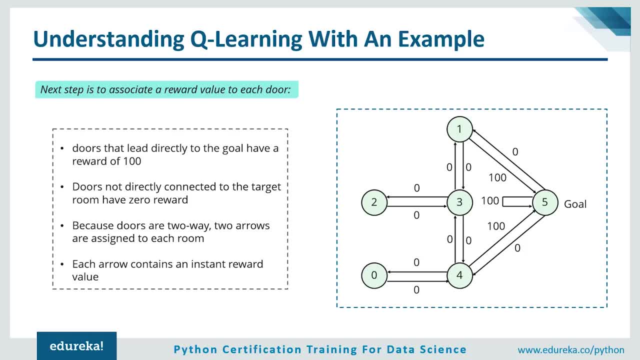 assigned to each room. So, basically, a zero leads to four and four leads back to zero. Now we've assigned zero over here because zero does not directly lead to five, but one directly leads to five, And that's why you can see that the two arrows are assigned to each room. So, basically, 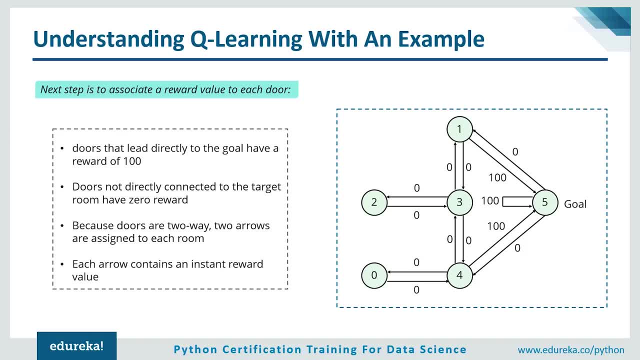 you can see a hundred over here. similarly, four directly leads to our goal state, and that's why we've assigned a hundred over here. and obviously five to five is hundred as well. so here all the direct connections to room number five are rewarded hundred and all the indirect connections. 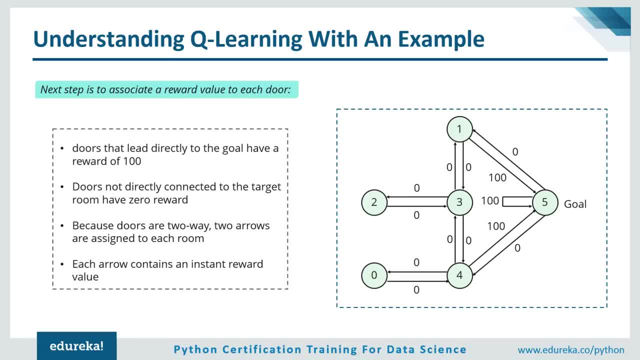 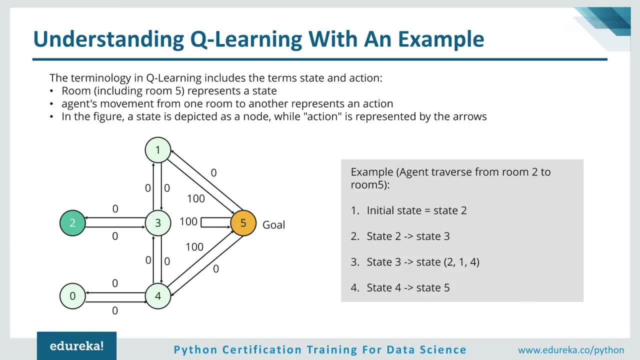 are rewarded zero. so, guys, in q learning, the end goal is to reach the state with the highest reward, so that the agent arrives at the goal. okay, so let me just explain this graph to you in detail now. these rooms over here labeled one, two, three to five. they represent the state an agent is in. 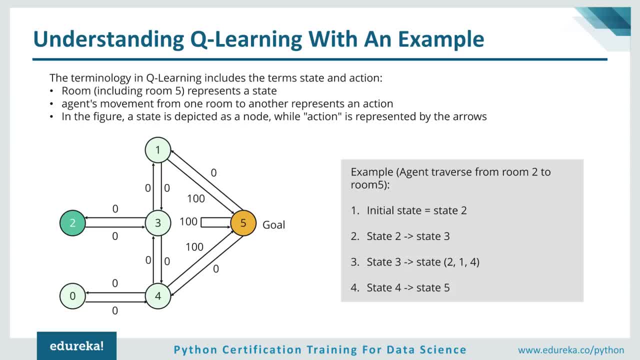 so if i state one, it means that the agent is in room number one. similarly, the agent's movement from one room to the other represents the action. okay, so if i say one, two, three, it represents an action, all right. so basically, the state is represented as node and the action is represented. 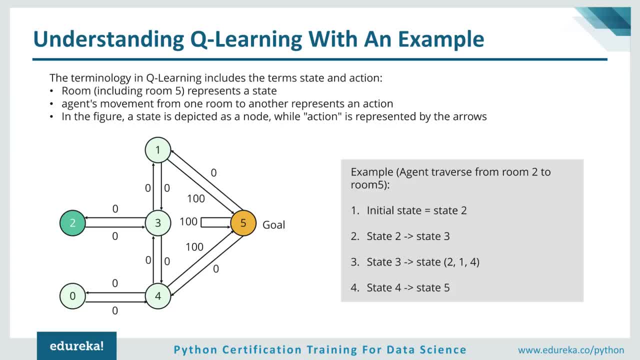 by these arrows. okay, so this is what this graph is about. these nodes represent the room and these arrows represent the actions. okay, let's look at a small example. let's set the initial state to zero, so my agent is placed in room number two and he has to travel all the way to room number. 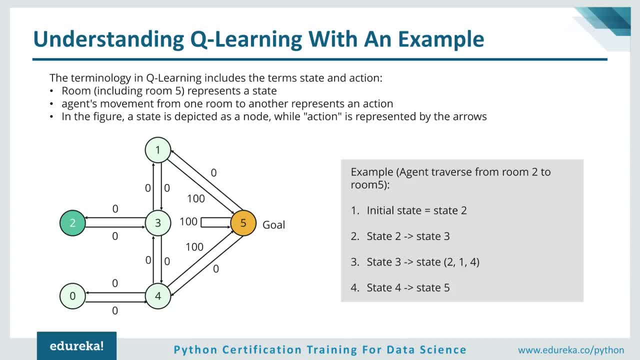 five. so if i set the initial stage to two, he can travel to state three. okay, from three he can either go to one, or he can go back to two, or he can go to four. if he chooses to go to four, it will directly take him to room number five. okay, which is our end goal. and even if he goes from room number three, 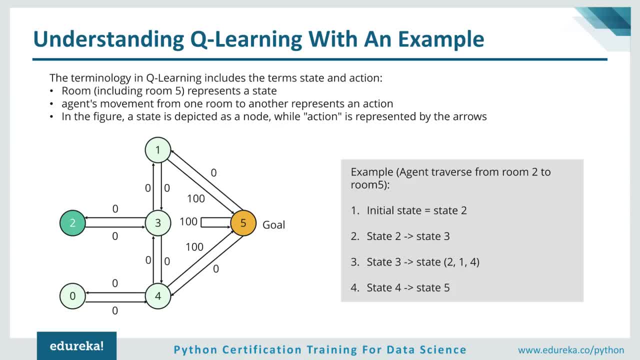 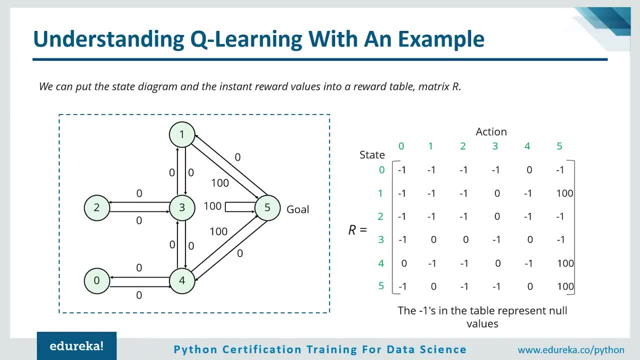 to one. he'll take him to room number five. so this is how our algorithm works. it's going to traverse different rooms in order to reach the goal room, which is room number five. now let's try and depict these rewards in the form of a matrix. okay, because we'll be using this r matrix, or the reward. 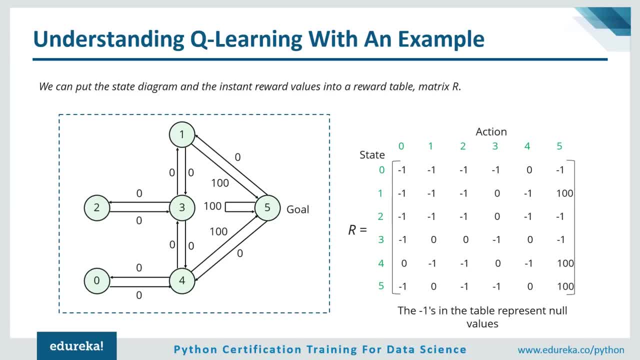 matrix to calculate the q value or the q matrix. okay, we'll see what the q value is in the next step, but for now let's see how this reward matrix is calculated. now, the minus ones that you see in the table. they represent the null values. now, these minus one: 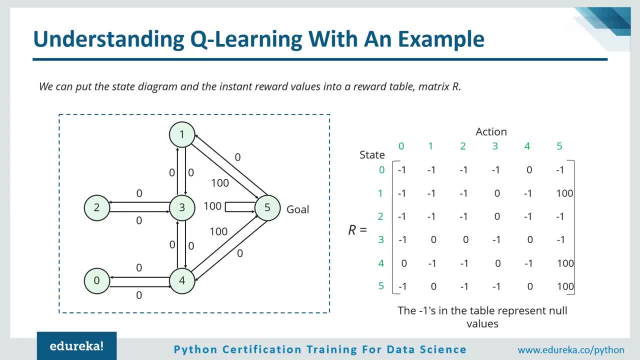 means that wherever there is no link between nodes, it's represented as minus one. so zero to zero is minus one. zero to one: there is no link. okay, there's no direct link from zero to one, so it's represented as minus one. similarly, zero to two, also, there is no link. you can see, there's no line. 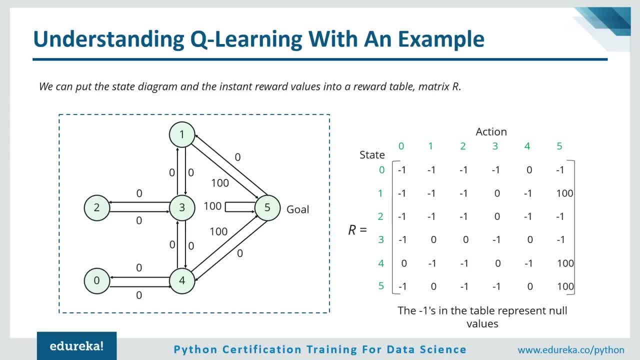 over here. so this is also minus one. but when it comes to zero to four, there is a connection and we have numbered it zero because the reward for a state which is not directly connected to the goal is zero. but if you look at this one of five, which is basically traversing from node one to node five, you can see the reward is hundred. 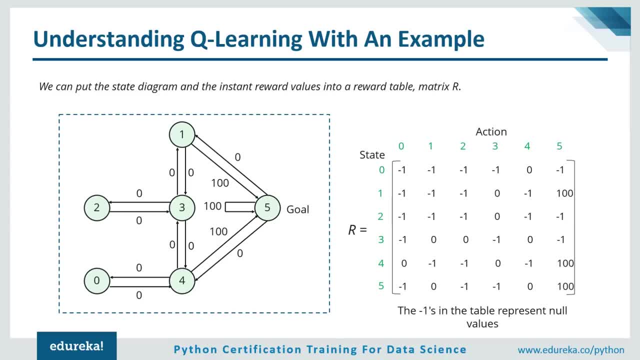 okay, that's basically because one and five are directly connected and five is our end goal. so any node which is directly connected to our goal state will get a reward of hundred. okay, that's why i've put hundred over here. similarly, if you look at the fourth row over here, i've assigned hundred. 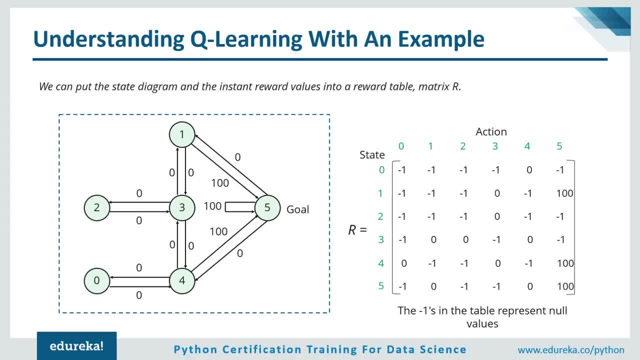 over here. this is because from four to five there is a direct connection, there's a direct connection which gives them a hundred reward. okay, you can see, from four to five there is a direct connection, a direct link. okay, so from room number four to room number five you can go directly. that's why 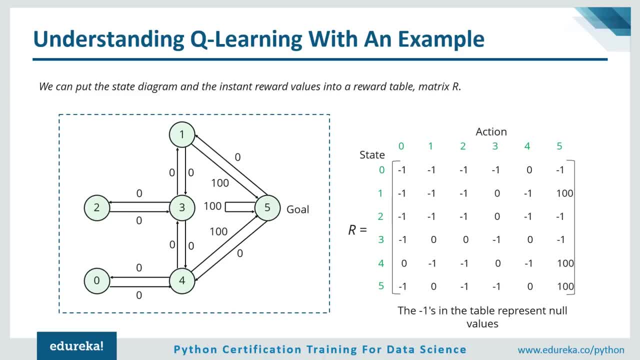 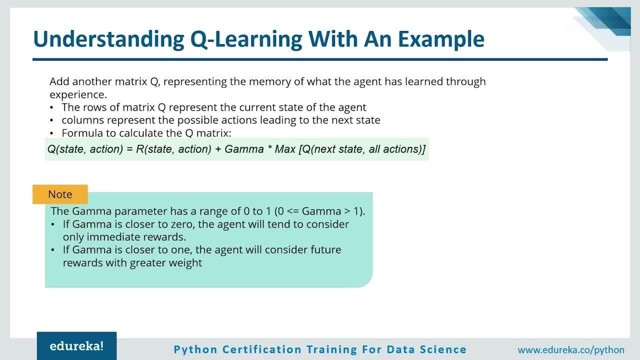 there's a hundred reward over here. so, guys, this is how the reward matrix is made. all right, i hope this is clear to y'all. okay, now that we have the reward matrix, we need to create another matrix called the q matrix. okay, here you'll store all the q values that we'll calculate now, this q matrix. 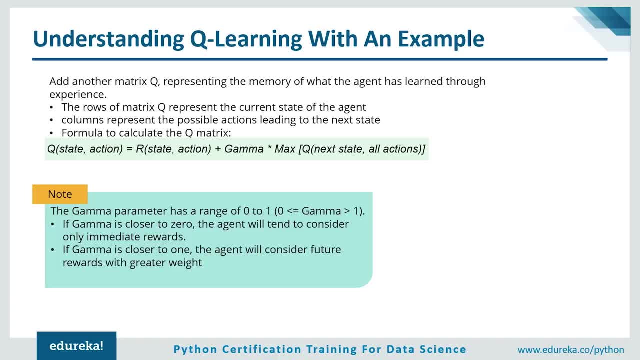 basically represents the memory of what the agent has learned through experience. okay, so once he traverses from one room to the final room, whatever the agent has learned through experience, whatever he's learned, is stored in this q matrix. okay, in order for him to remember that the next. 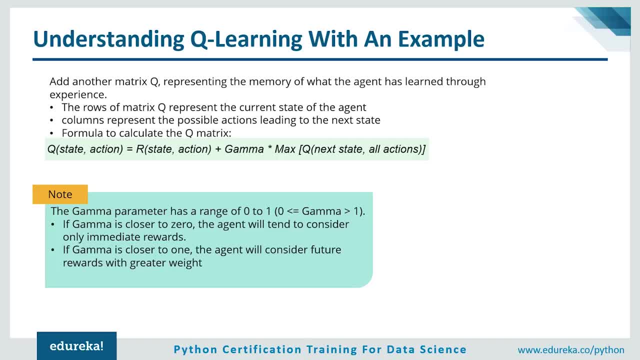 time he traverses. we use this matrix. okay, it's basically like a memory. so, guys, the rows of the q matrix will represent the current state of the agent, the columns will represent the possible actions and to calculate the q value, you use this formula. all right, i'll show you what the q matrix. 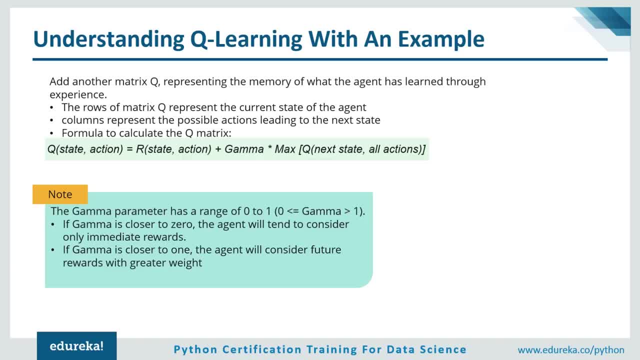 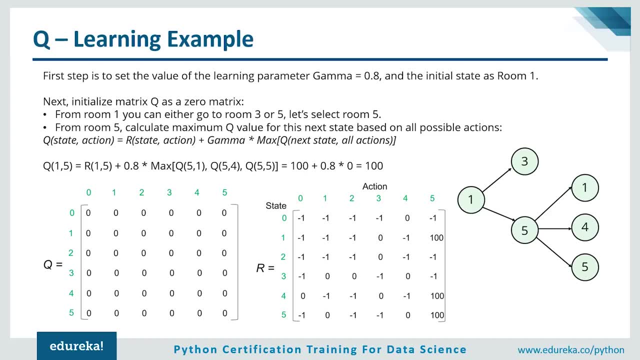 looks like. but first let's understand this formula. now, this q value we're calculating because we want to fill in the q matrix. okay, so this is basically a q matrix. over here. initially it's all zero, but as the agent traverses from different nodes to the destination node, this matrix will get filled up. okay, so basically it'll. 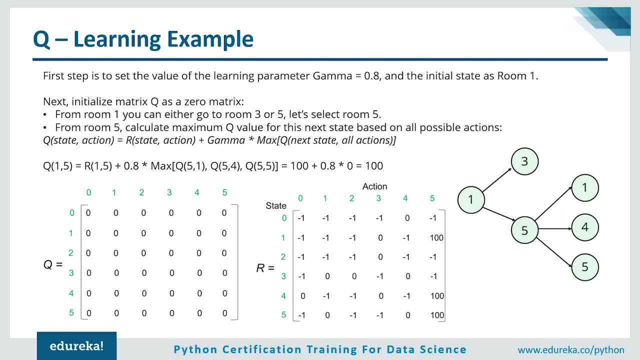 be like a memory to the agent. he'll know that. okay, when he traversed using a particular path, he found out that his value was maximum or his reward was maximum over here, so next time he'll choose that path. this is exactly what the q matrix is. okay, let's go back now. guys, don't worry about. 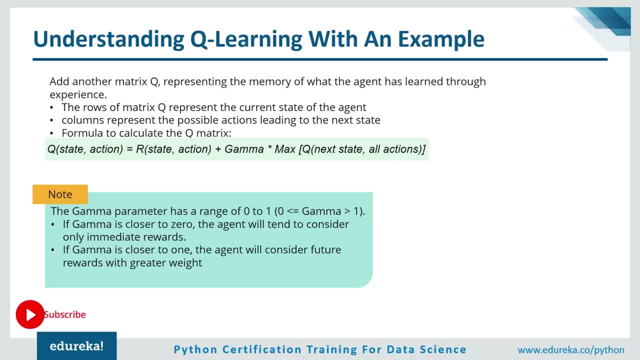 this formula for now, because we'll be implementing this formula in a different way, in a different way. an example in the next slide. okay, so don't worry about this formula for now, but here, just remember that this q basically represents the q matrix, the r represents the reward matrix and the gamma is the 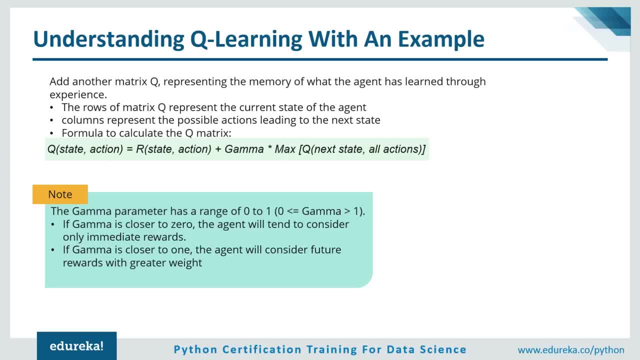 gamma value, which i'll talk about shortly, and here you're just finding out the maximum from the q matrix. so basically, the gamma parameter has a range from zero to one. so you can have a value of 0.1, 0.3, 0.5, 0.8, and all of that so if the gamma is closer to. 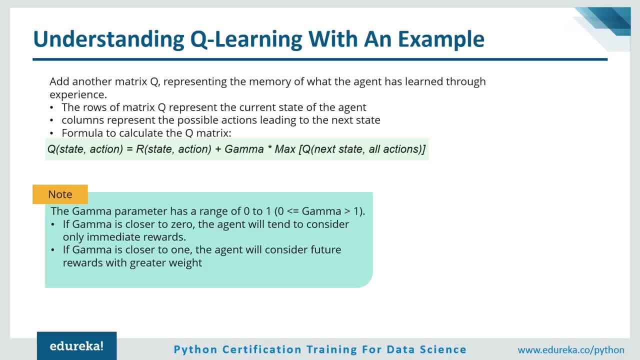 zero, it means that the agent will consider only the immediate rewards, which means that the agent will not explore the surrounding. basically, it won't explore different rooms, it'll just choose a particular room and then it'll try sticking to it. but if the value of gamma is high, meaning that 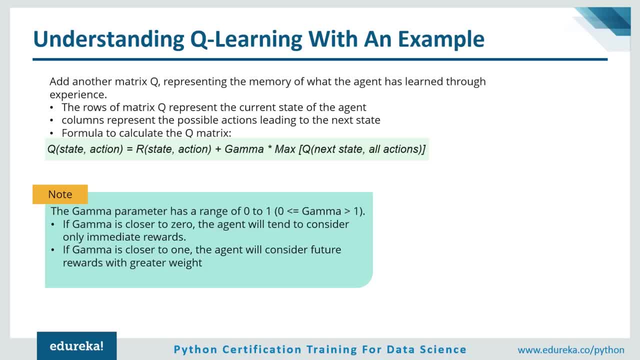 if it's closer to one, the agent will consider future rewards with greater weight. this means that the agent will explore all the possible approaches or all the possible policies in order to get to the end goal. so, guys, this is what i was talking about when i mentioned exploitation and exploration. all right, so if the gamma value is closer to one, 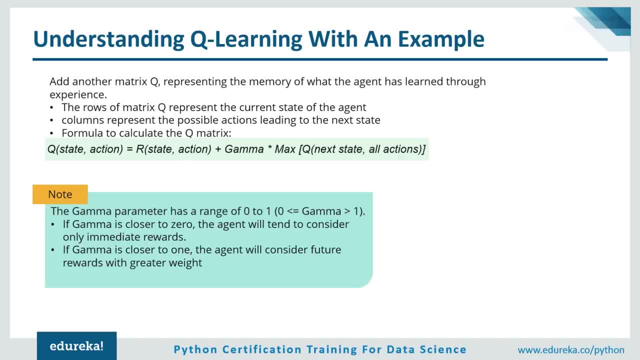 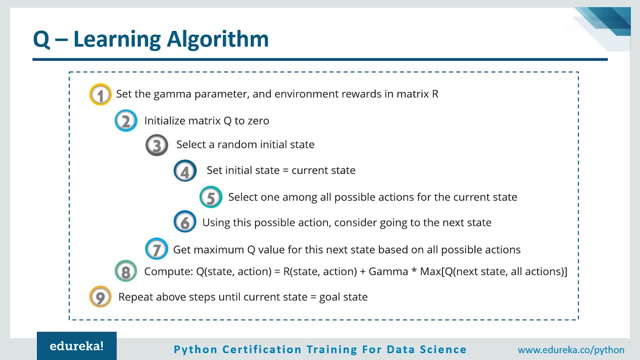 it basically means that you're actually exploring the entire environment and then choosing an optimum policy. but if your gamma value is closer to zero, it means that the agent will only stick to a certain set of policies and it will calculate the maximum reward based on those policies. now, next, we have 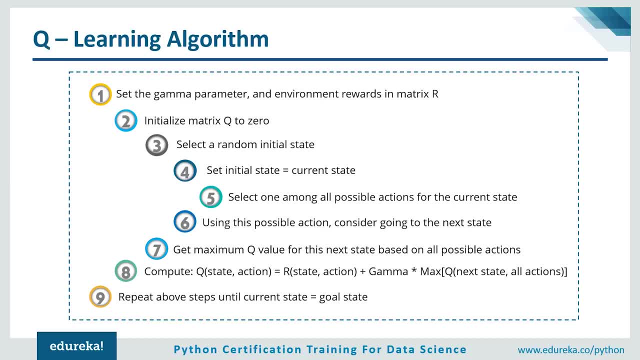 the q learning algorithm that we're going to use to solve this problem. so, guys, now this is going to look very confusing to y'all, so let's start with the q learning algorithm, and we're going to explain this with an example. okay, we'll see what we're actually going to run in our demo. we'll do. 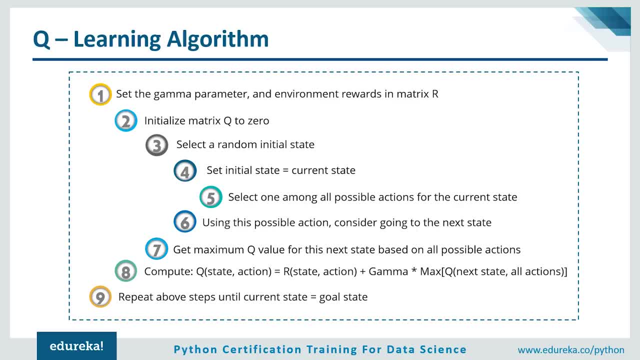 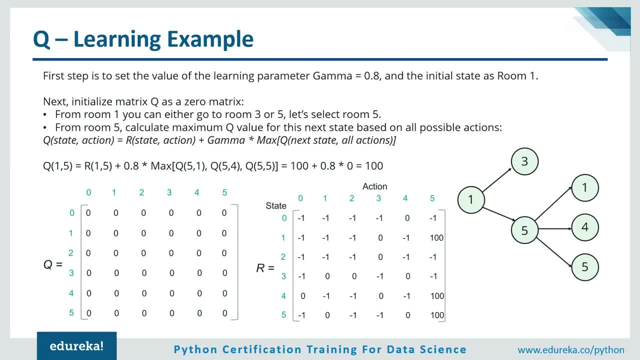 the math behind it, and then i'll tell you what this q learning algorithm is. okay, you'll understand it, as i'm showing you the example. so, guys, in the q learning algorithm, the agent learns from his experience. okay, so, each episode, which is basically when the agent starts traversing from an initial 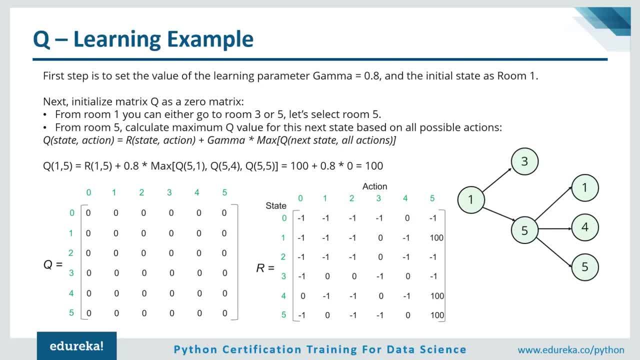 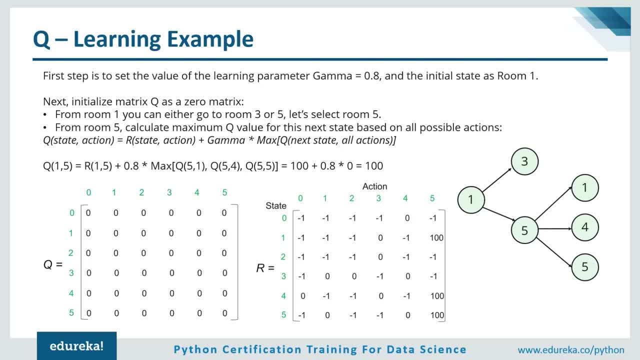 purpose of training is to enhance the brain of our agent. okay, only if he knows the environment very well will he know which action to take. and this is why we calculate the q matrix. okay, in q matrix, which is going to calculate the value of traversing from every state to the end state, from every 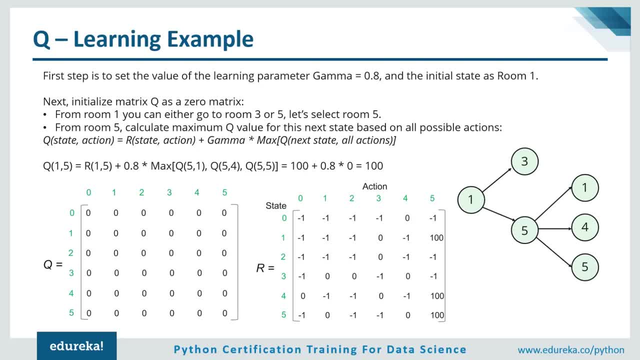 initial room to the end room. okay. so when we calculate all the values, or how much reward we're going to get, we know the policy that we take. we know the optimum policy that will give us the maximum reward. okay, that's why we have the q matrix. this is very important because the more you train, 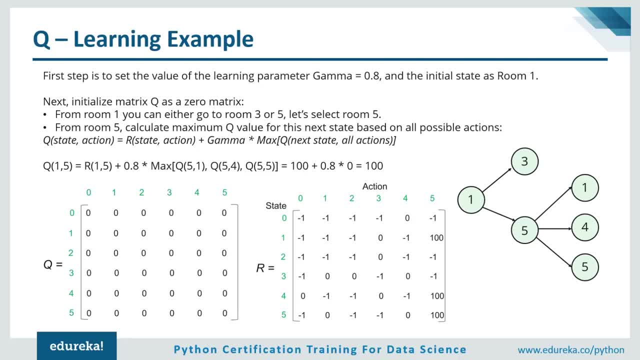 the agent and the more optimum your output will be. so, basically, here, the agent will not perform exploitation. instead, he'll explore around and go back and forth through the different rooms and find the fastest route to the goal. all right, now let's look at an example. okay, let's see how the 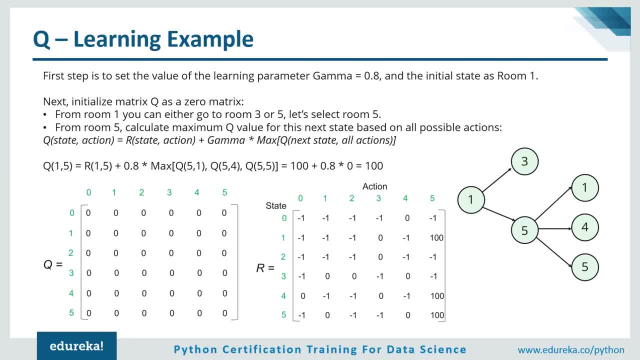 algorithm works. okay, let's go back to the previous slide, and here it says that the first step is to set the gamma parameter. okay, so let's do that now. the first step is to set the value of the learning parameter, which is gamma, and we've randomly set. 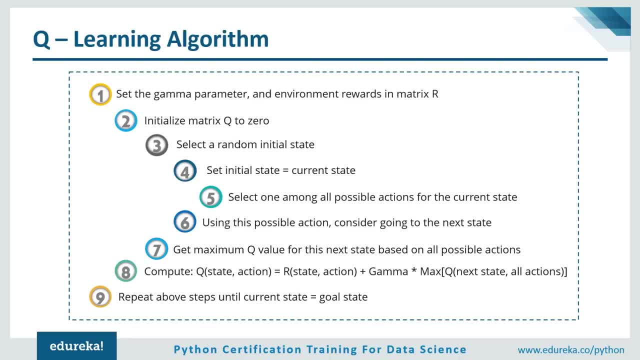 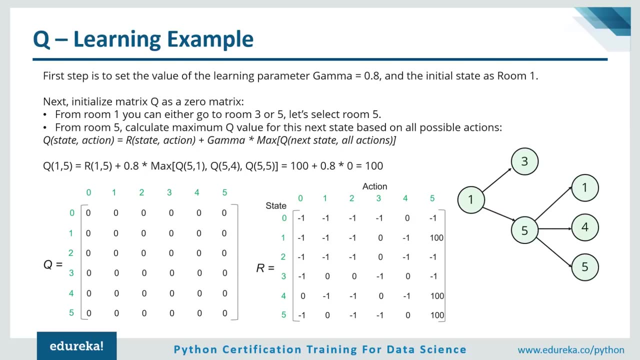 it to 0.8. okay. the next step is to initialize the matrix q to zero. okay, so we've set matrix q to zero over here, and then we'll select the initial stage. okay. the third step is select a random initial state, and here we've selected the initial state as room number one. okay, so after you. 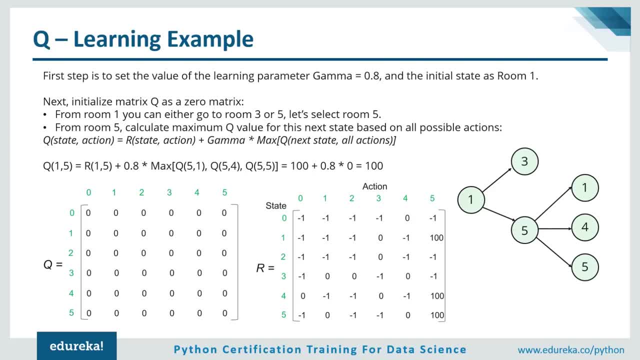 initialize the matrix q as a zero matrix. from room number one you can either go to room number three or room number five. so if you look at the reward matrix you can see that from room number one you can only go to room number three or room number five. the other values are minus one here, which 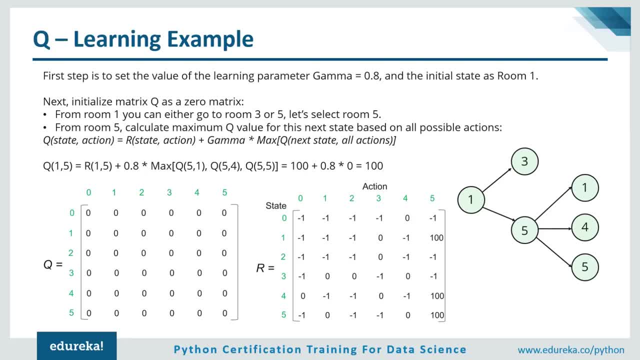 means that there is no link from one to zero, one to one, one to two and one to four, so the only possible actions from room number one is to go to room number three and to go to room number five. all right, okay, so let's select room number. 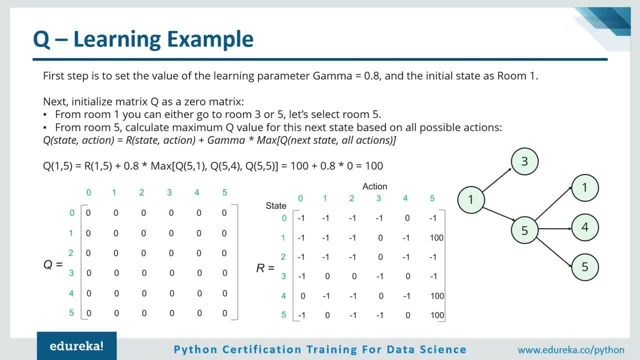 five. okay, so from room number one you can go to three and five, and we have randomly selected five. you can also select three, but for example, let's select five over here. now, from room five, you're going to calculate the maximum q value for the next state based on all possible actions. so from 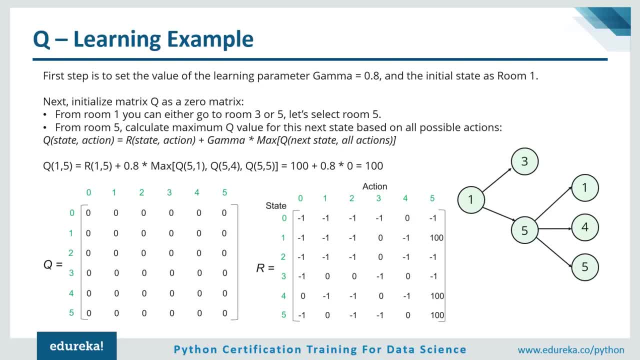 room number five. the next state can be room number one, four or five. so you're going to calculate the q value for traversing five to one, five to four, five to five, and you're going to find out which has a maximum q value. that's how you're going to compute the q value. so let's implement our formula. okay, this is the 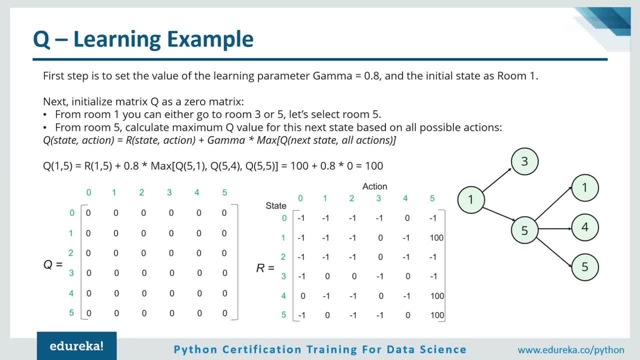 q learning formula. so right now we're traversing from room number one to room number five. okay, this is our state. so here i've written q, one comma five. okay, one represents our current state, which is room number one. okay, our initial state was room number one and we are traversing to room number. 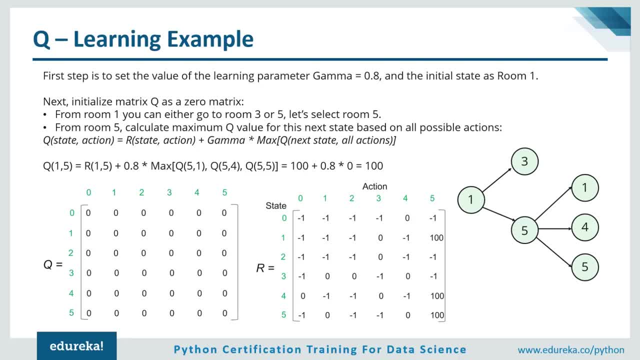 five. okay, it's shown in this figure, room number five. now for this we need to calculate the q value. next, in our formula it says reward matrix, state and action. so the reward matrix for one comma five. let's look at one comma five. one comma five corresponds to hundred. okay, so our reward over here will be hundred. so r one comma five is basically. 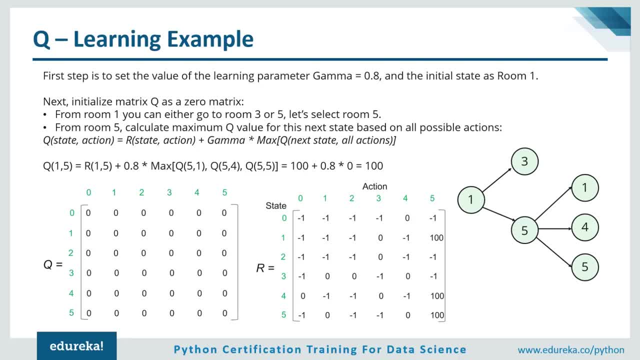 hundred, then you're going to add the gamma value. now, the gamma value, we've initialized it to 0.8, so that's what we've written over here, and we're going to multiply it with the maximum value that we're going to get for the next state, based on all possible actions. okay, so from five the next. 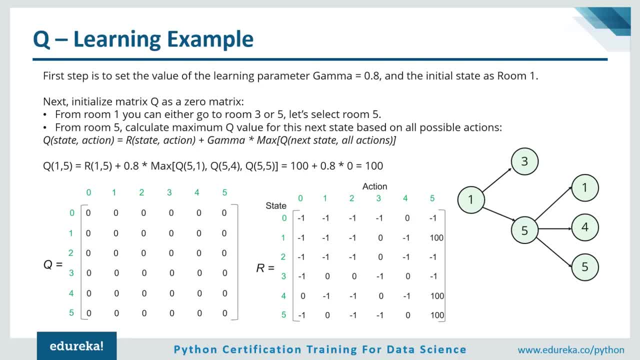 state is one, four and five, and we're going to add the gamma value to the next state, based on all possible actions. okay, so if you traverse from five to one- that's what i've written over here- five to four- you're going to calculate the q value of five to four and five to five. okay, that's what. 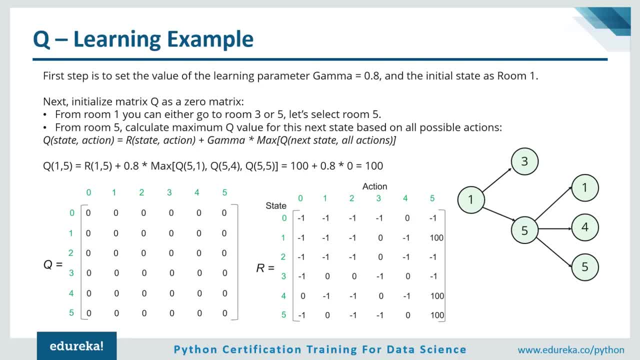 i mentioned over here. so q five comma one, five comma four and five comma five are the next possible actions that you can take from state five. so r one comma five is hundred. okay, because from the reward matrix you can see that one comma five is hundred. 0.8 is the value of gamma. after that, 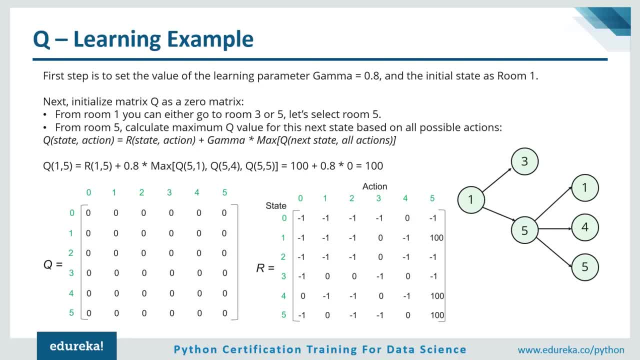 we'll calculate q of five comma one, five comma four and five comma five and we're going to add one comma five. like i mentioned earlier that we're going to initialize matrix q as zero matrix. so we're setting the value as zero because initially obviously the agent doesn't have any. 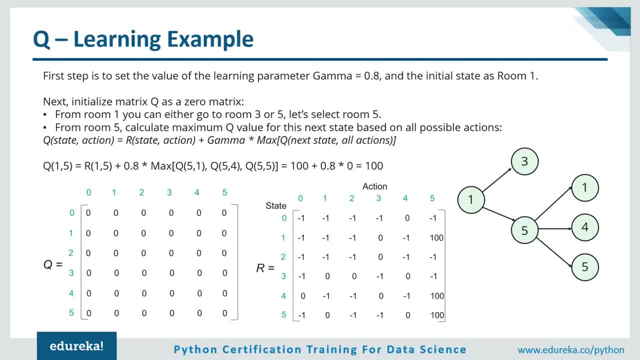 memory of what is happening. okay, so he's just starting from scratch. that's why all these values are zero. so q of five comma one will obviously be zero, five comma four will be zero and five comma five will also be zero. and to find out the maximum between these, it's obviously zero. 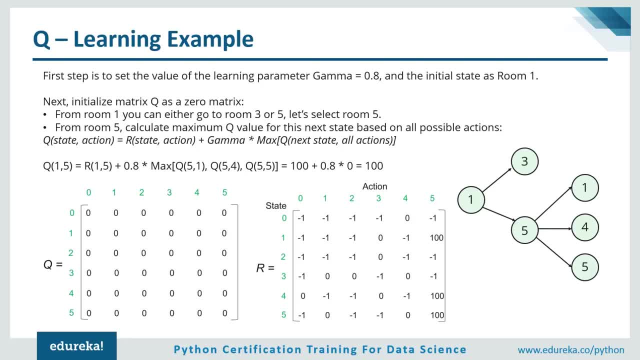 so when you compute this equation you'll get hundred. so the q value of one comma five is hundred. so if our agent goes from room number one to room number five, he's going to have a maximum reward or q value of hundred. all right now in the next slide you can see that i've updated. 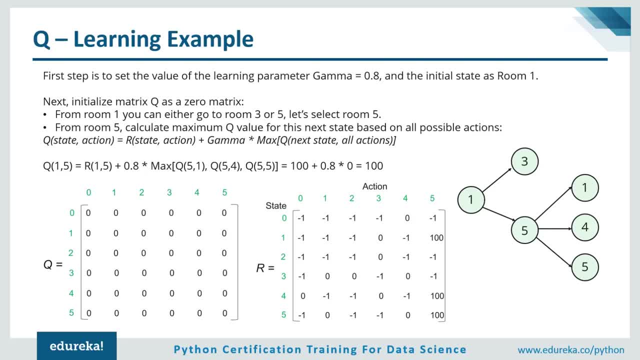 the value of q of one comma five. okay, it's set to hundred, all right now. similarly, let's look at another example so that you understand this better. so, guys, this is exactly what we're gonna do in our demo. it's only going to be coded. okay, i'm just explaining our code right now. i'm just telling. 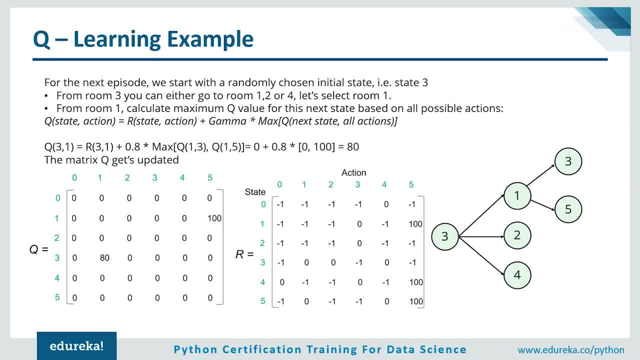 you the math behind it. all right, let's look at another example. okay, this time we'll start with a randomly chosen initial state. let's say that we've chosen state three. okay, so from room three, you can either go to room number one, two or four randomly. we'll select room number one and from room number one you're going to. 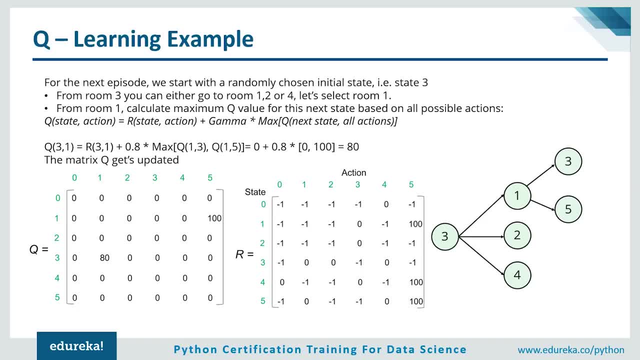 calculate the maximum q value for the next state based on all possible actions. so the possible actions from one is to go to three and to go to five. now, if you calculate the q value using this formula, so let me explain this to you once again now. q three comma one basically represents that we are in room number three. 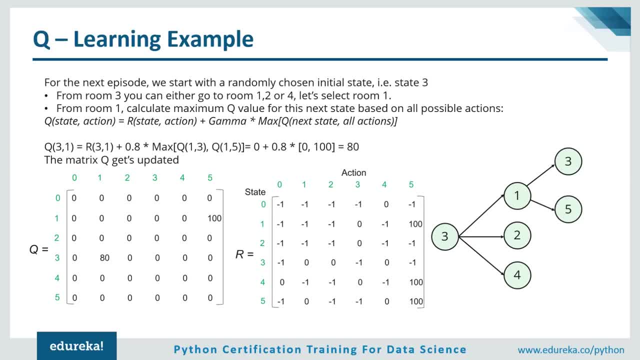 and we are going to room number one. okay, so this represents our action. okay, so we're going from three to one, which is our action, and three is our current state. next you'll look at the reward of going from three to one. okay, if you go to the reward, matrix three, comma one is zero. okay, now. 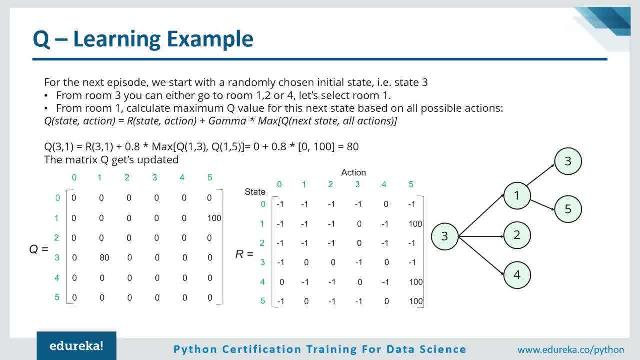 this is because there's no direct link between three and five. okay, so that's why the reward here is zero, so the value here will be zero. after that we have a gamma value which is zero point eight, and then we're going to calculate the q max of one comma three and one. 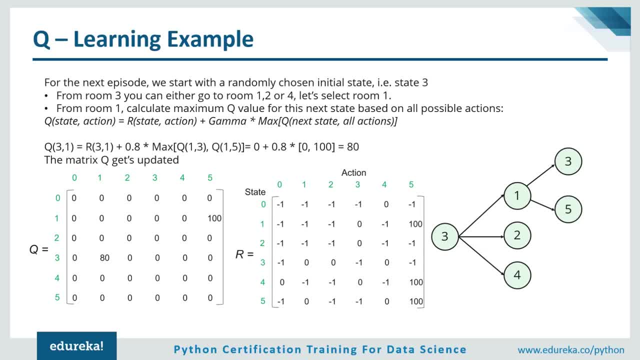 comma five out of these, whichever has the maximum value, we're going to use that. okay, so q of one comma three is zero. all right, it's zero. you can see here: one comma three is zero and one comma five. if you remember, we just calculated one comma five in the previous slide. okay, one comma five is 100. 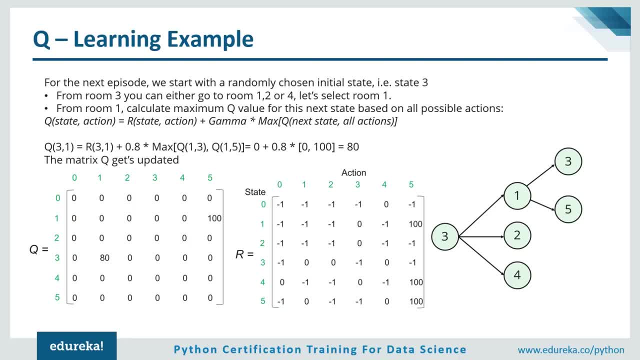 so here i'm going to put 100. so, uh, the maximum here is 100, so 0.8 into 100 will give us 80.. so that's the q value we are going to get if you traverse from three to one. okay, i hope that was clear. 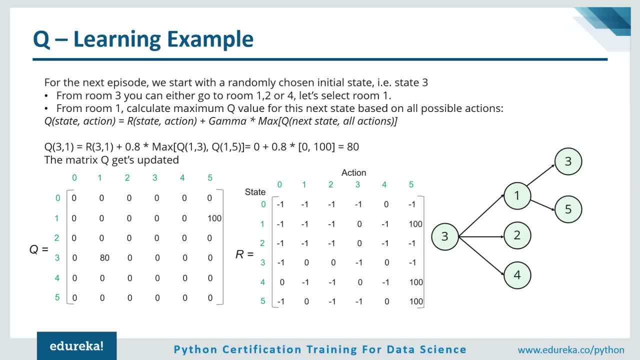 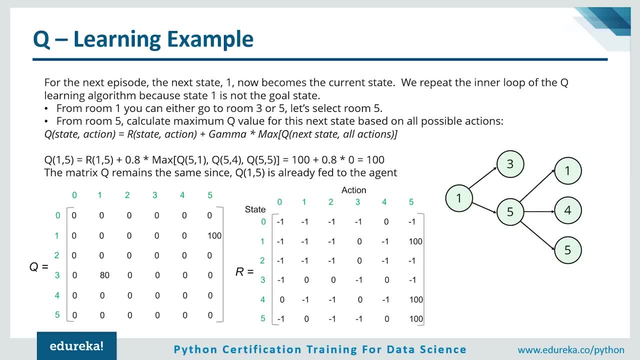 so now we've traversed from room number three to room number one with a reward of 80.. okay, but we still haven't reached the end goal, which is room number five. so for our next episode, the state will be room number one. so, guys, like i said, we'll repeat this. 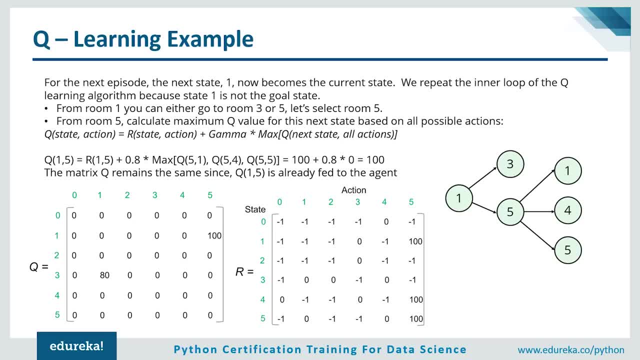 in a loop because room number one is not our end goal. okay, our end goal is room number five. so now we need to figure out how to get from room number one to room number five. Room number one: you can either go to three or five. 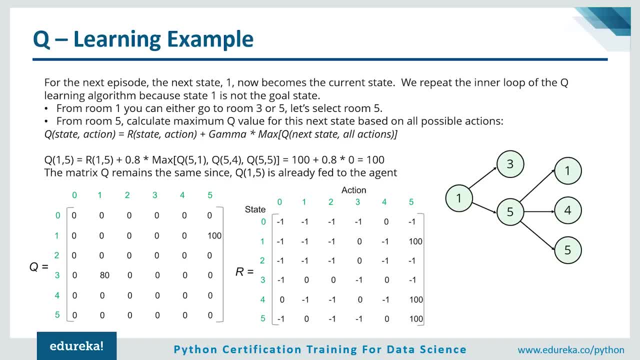 That's what I've drawn over here. So if we select five, we know that it's our end goal, okay. So from room number five, then you have to calculate the maximum Q value for the next possible actions. So the next possible actions from five. 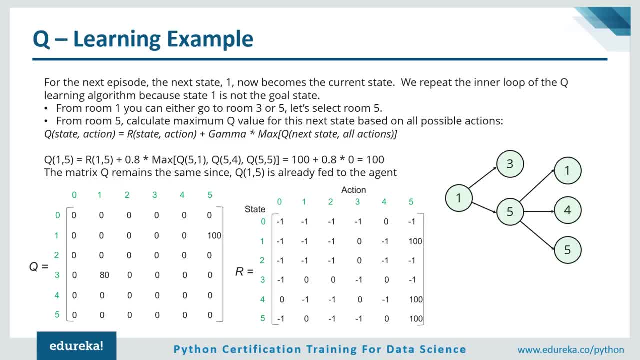 is to go to room number one, room number four or room number five. So you're going to calculate the Q value of five to one, five to four and five to five and find out which is the maximum Q value here. 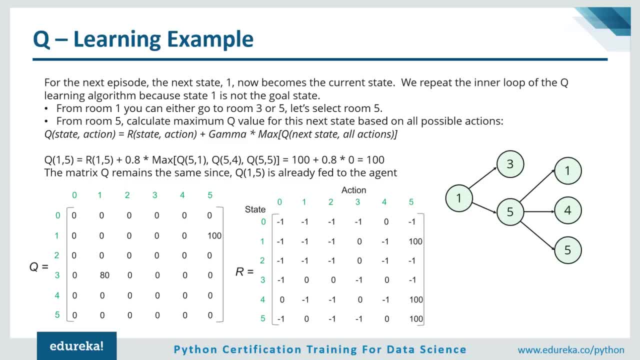 and you're going to use that value. all right, So let's look at the formula now. Now again, we're in room number one and we want to go to room number five. okay, So that's exactly what I've written here: Q one comma five. 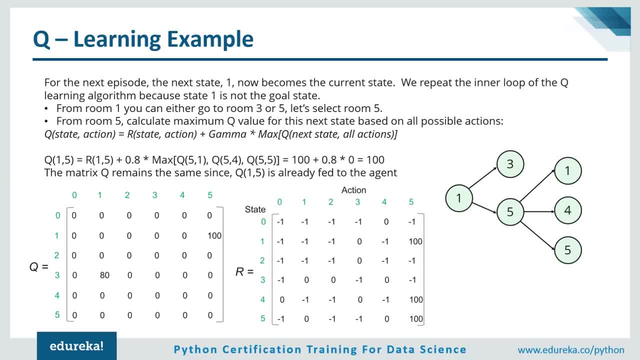 Next is the reward matrix, so reward of one comma five, which is 100,. all right, Then we've added the gamma value, which is 0.8, and then we're going to find the maximum Q value from five to one, five to four and five to five. 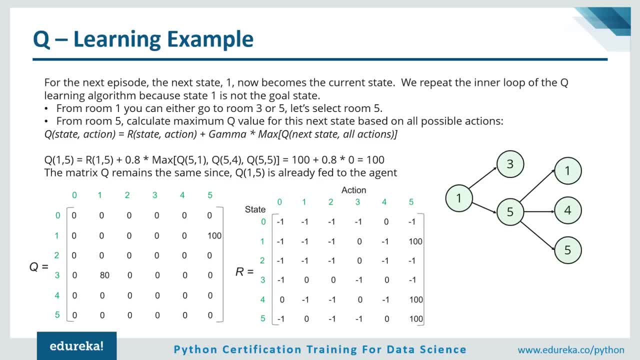 So this is what we're performing over here. So five comma one, five comma four and five comma five are all zero. This is because we initially set all the values of the Q value and we're going to add the Q matrix as zero. 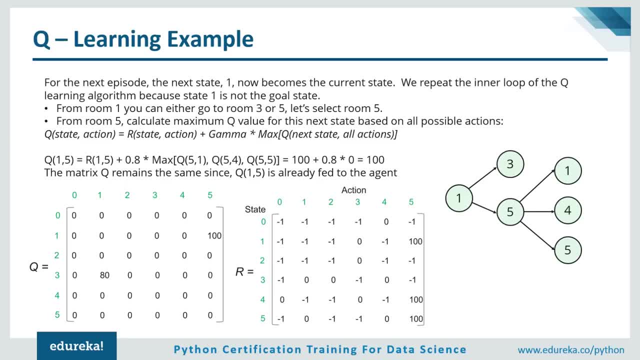 So you get 100 over here and the matrix remains the same, because we already had calculated Q one comma five. So the value of one comma five is already fed to the agent. So when he comes back here he knows that okay. 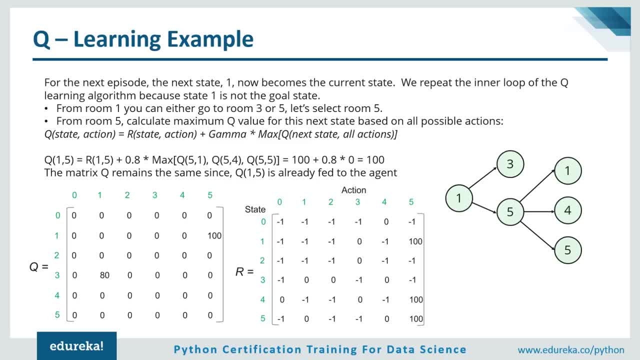 he's already done this before. Now he's going to try and implement another method. okay, He's going to try and take another route or another policy. So he's going to try to go from different rooms and finally land up in room number five. 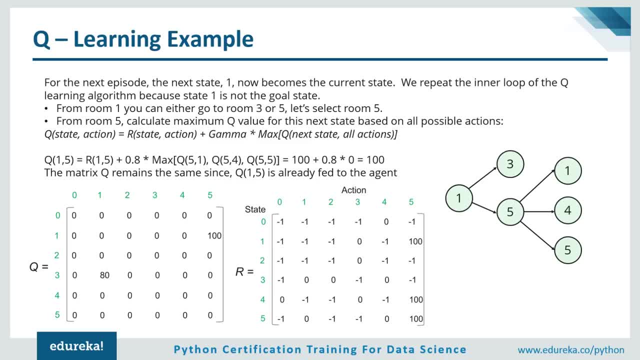 So, guys, this is exactly how our code runs. We're going to traverse through each and every node Because we want an optimum policy. okay, An optimum policy is attained only when you traverse through all possible actions. okay, So if you go through all possible actions, 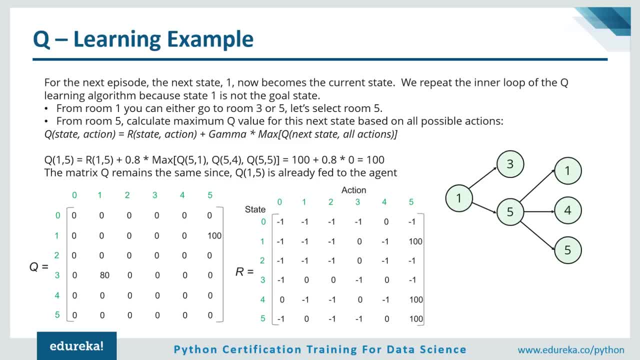 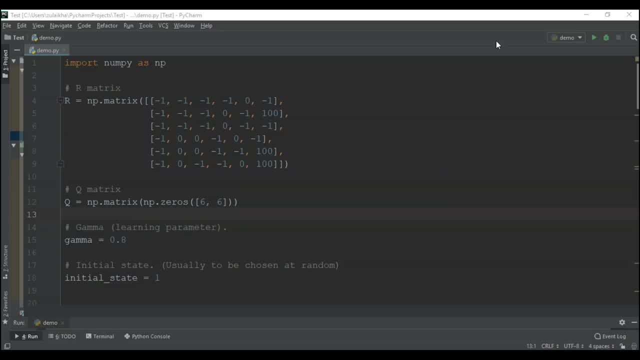 that you can perform. only then will you understand which is the best action which will lead us to the reward. I hope this is clear. Now let's move on and look at our code. So, guys, this is our code and this is executed in Python. 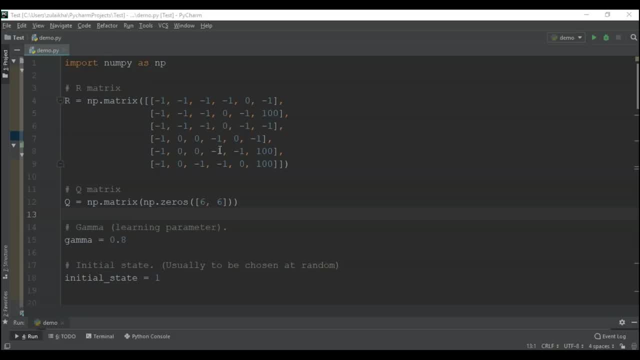 and I'm assuming that all of you have a good background in Python. okay, If you don't understand Python very well, I'm going to leave a link in the description. You can check out that video on Python and then maybe come back to this later. okay, 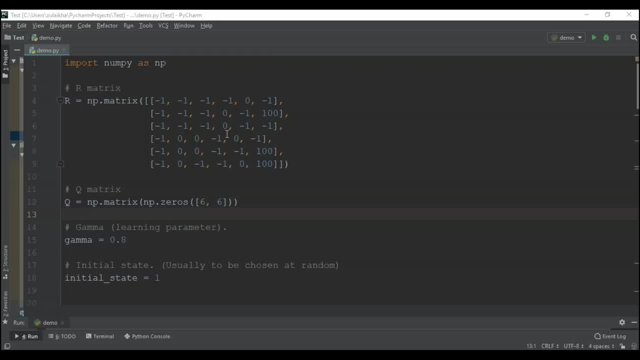 But I'll be explaining the code to you anyway. but I'm not going to spend a lot of time explaining each and every line of code, because I'm assuming that you know Python, okay, So let's look at the first line of code over here. 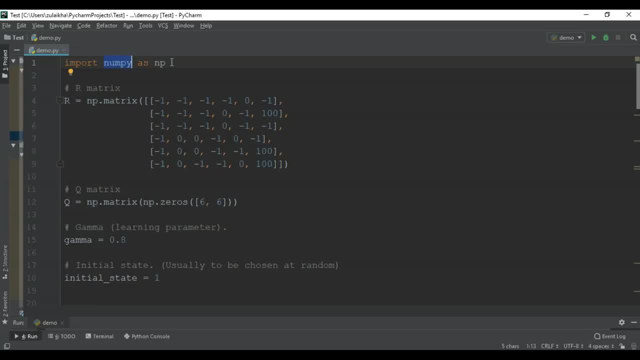 So what we're going to do is we're going to import numpy. okay, Numpy is basically a Python library for adding support for large multidimensional arrays and matrices and it's basically for computing mathematical functions. okay, So first we're going to import that. 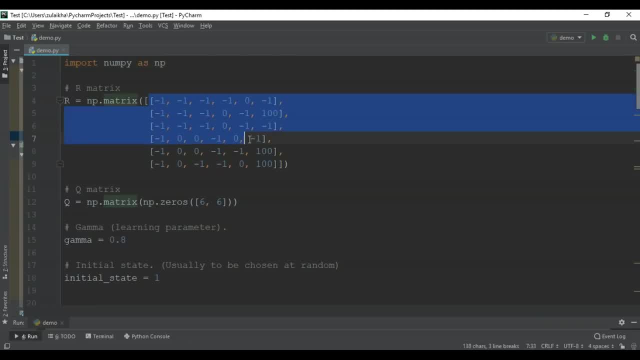 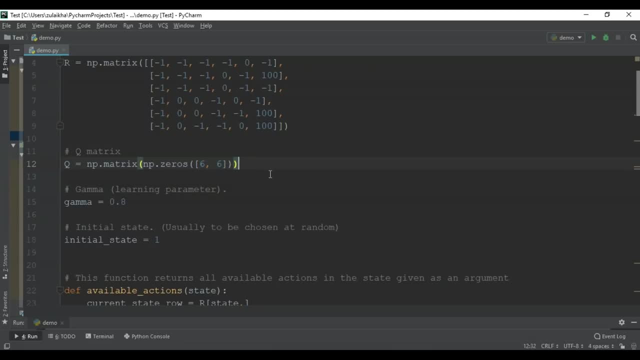 After that, we're going to create the R matrix. okay, So this is the R matrix. Next, we're going to create a Q matrix, and it's a six into six matrix, because obviously we have six states starting from zero to five. okay, 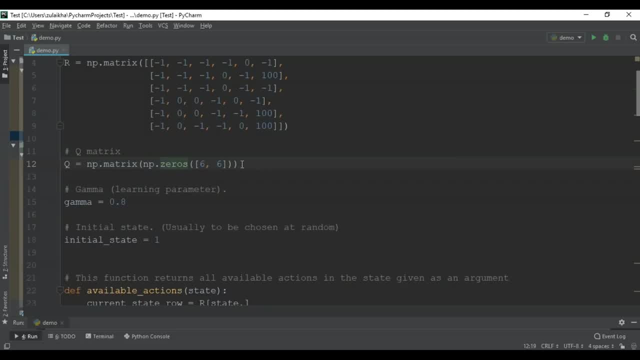 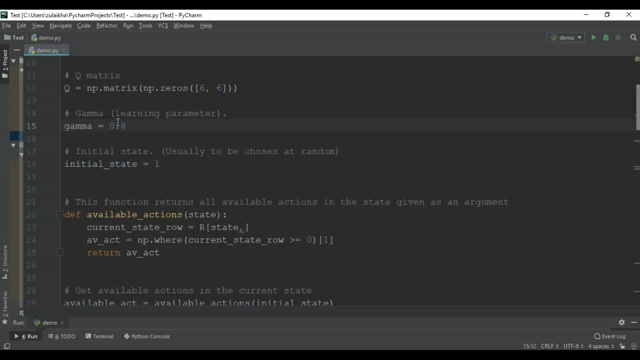 And we're going to initialize the value to zero. So, basically, the Q matrix is going to be initialized to zero over here, all right. After that we're setting the gamma parameter to 0.8.. So, guys, you can play with this parameter. 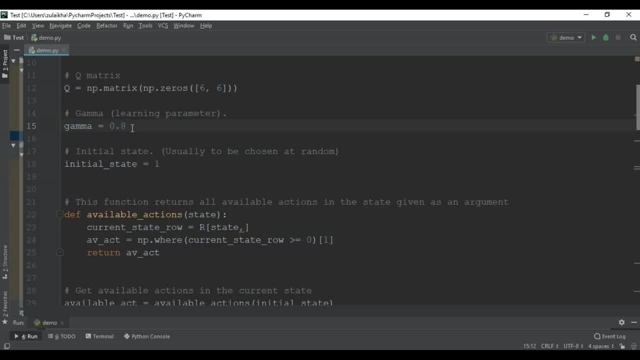 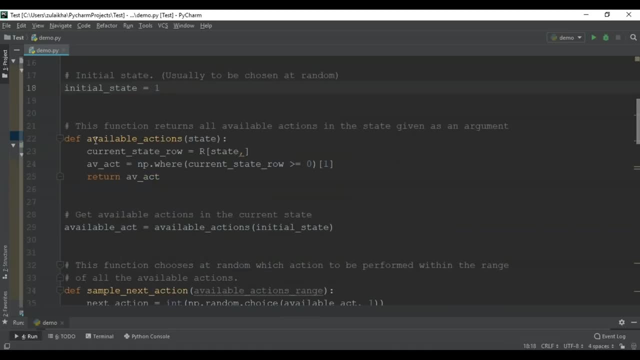 and move it to 0.9.. Or move it lower to 0.8,. okay, You can see what happens then. Then we'll set an initial stage. okay, Initial stage is set as one. After that, we're defining a function. 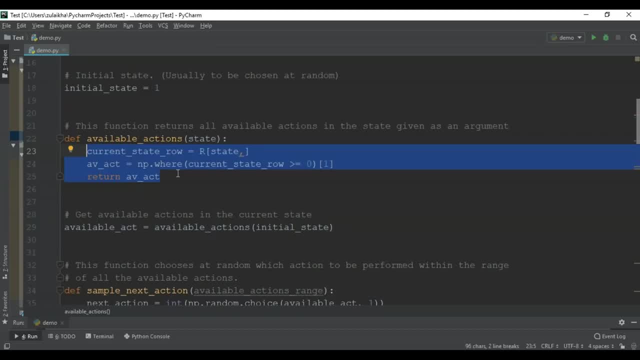 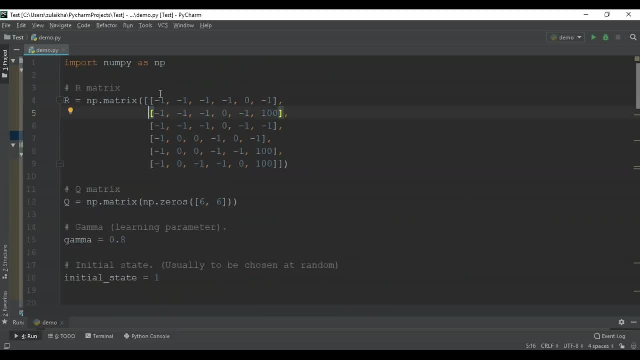 called available actions, okay. So basically, what we're doing here is, since our initial state is one, we're going to check our row number one. okay, This is our row number one. okay, This is row number zero, This is row number one, and so on. 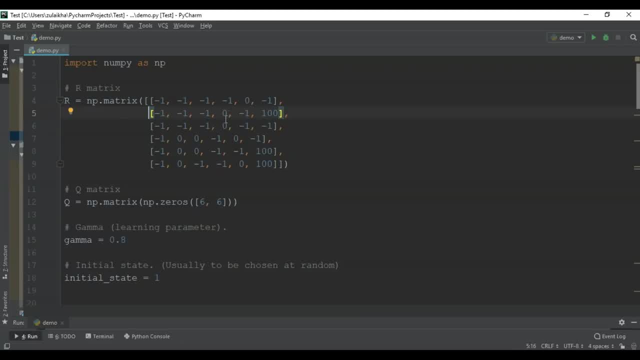 So we're going to check the row number one and we're going to find the values which are greater than or equal to zero, Because these values basically represent the nodes that we can travel to. Now, if you select minus one, you can't traverse to minus one. okay, 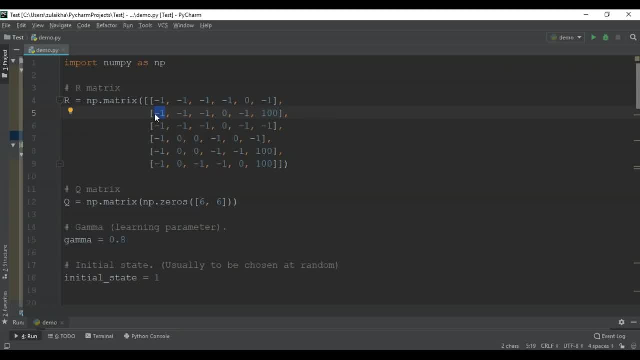 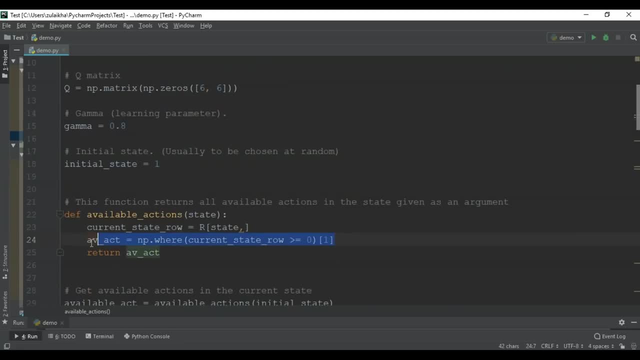 I explained this earlier. The minus one represents all the nodes that we can't travel to, But we can travel to these nodes, okay? So basically, over here we're checking all the values which are equal to zero or greater than zero. 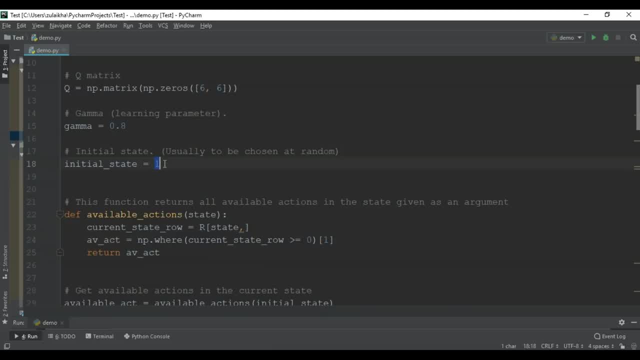 These will be our available actions. So if our initial state is one, we can travel to other states whose value is equal to zero or greater than zero, And this is stored in this variable called available act. all right, Now, this will basically get the available actions. 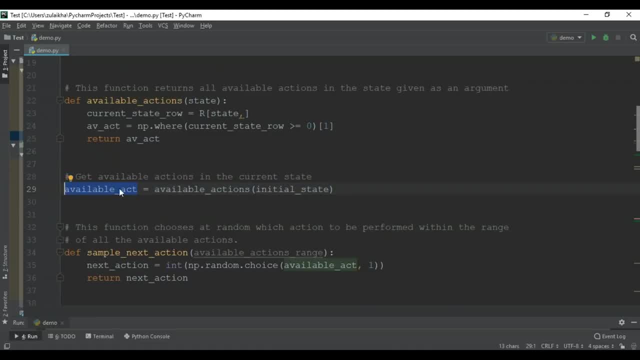 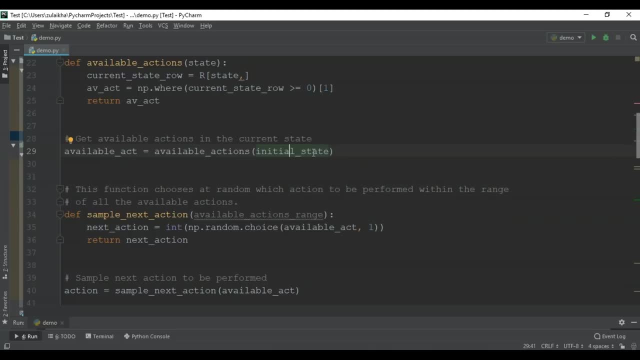 in the current state. okay, So we're just storing the possible actions in this available act variable over here. So basically over here, since our initial state is one we're going to find out the next possible states we can go to. okay. 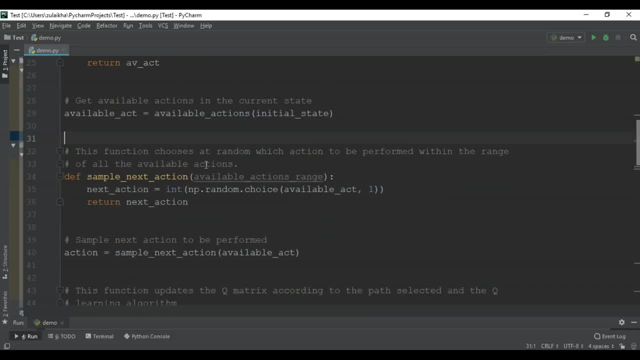 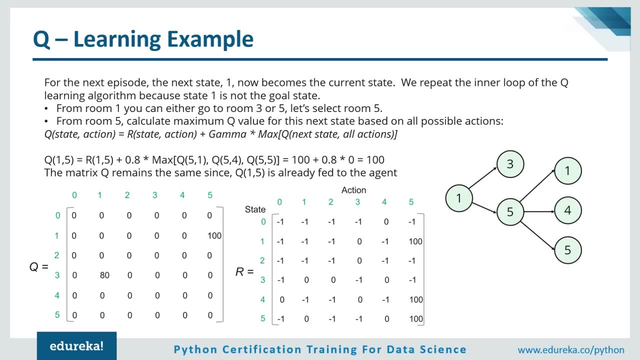 That is stored in the available act variable. Now next is this function chooses at random which action to be performed within the range. So, if you remember over here. so, guys, initially we are in stage number one. okay, Our available actions is to go to stage number three. 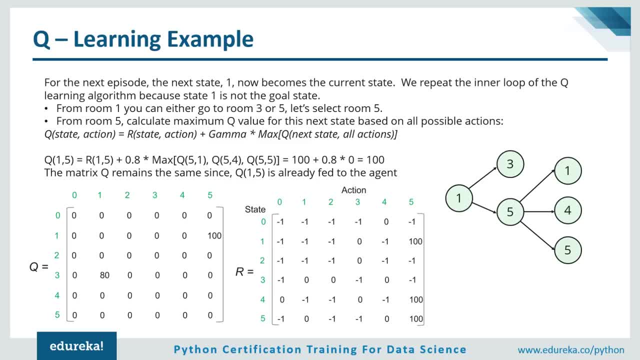 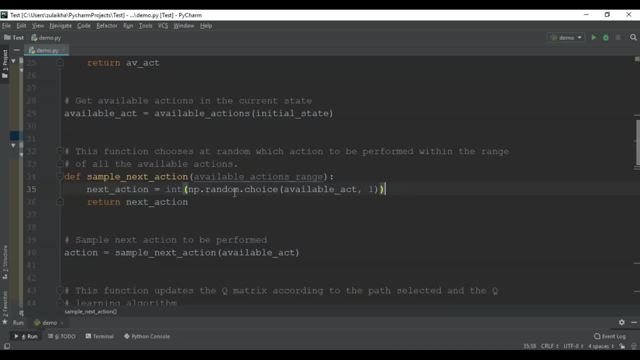 or stage number five, Sorry, room number three or room number five. Okay, now, randomly, we need to choose one room, So for that we're using this line of code. okay, So here we're randomly going to choose one of the actions. 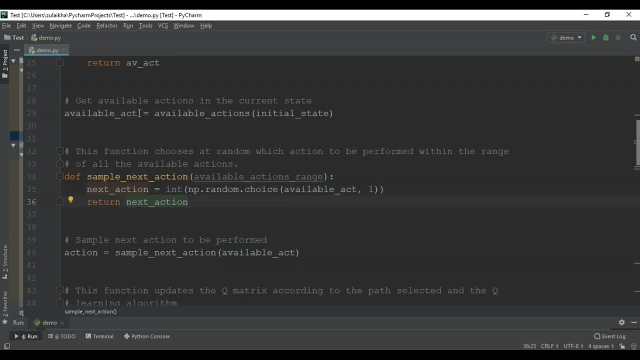 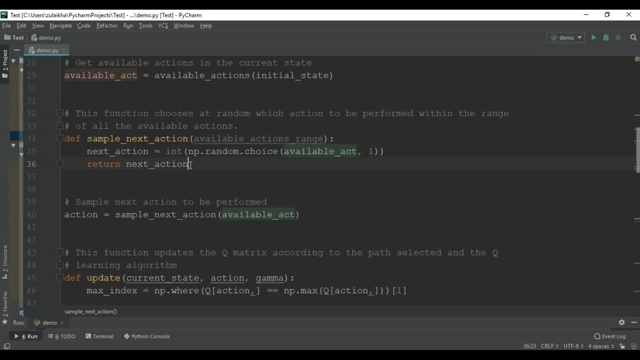 from the available act. This available act, like I said earlier, stores all our possible actions, okay, from the initial state. okay. So once it chooses an action, it's going to store it in next action. So, guys, this action will represent. 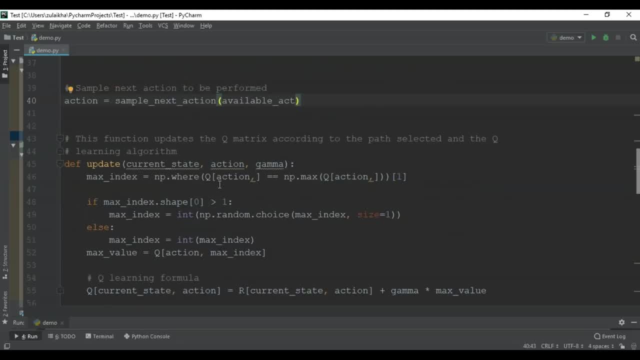 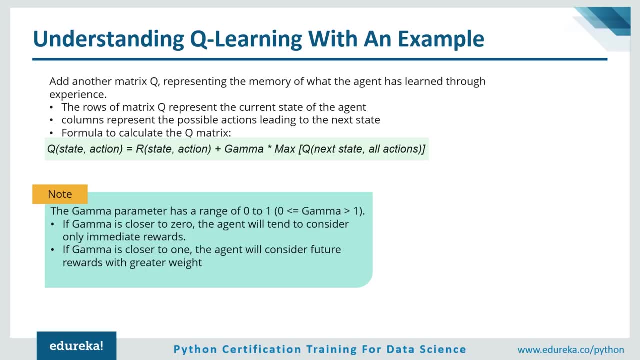 the next available action to take Now. next is our Q matrix. Remember this formula that we used? So, guys, this formula that we use is what we're going to calculate in the next few lines of code, So in this block of code. 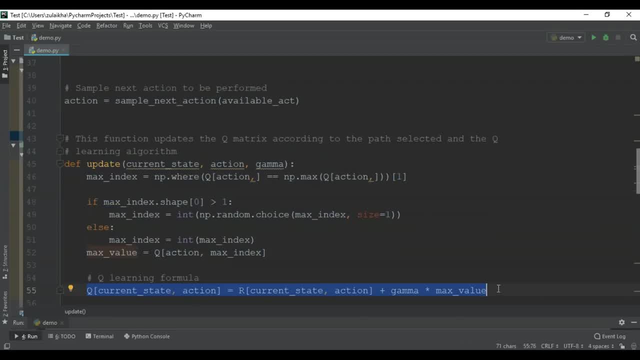 we're just executing and computing the value of Q. okay, This is our formula for computing the value of Q, current state comma action, our current state comma action, gamma into the maximum value. So here, basically, we're going to calculate. 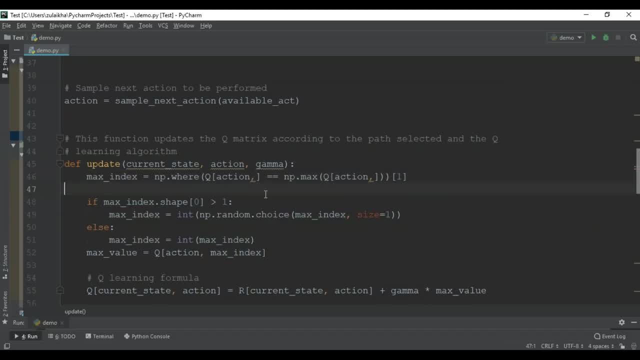 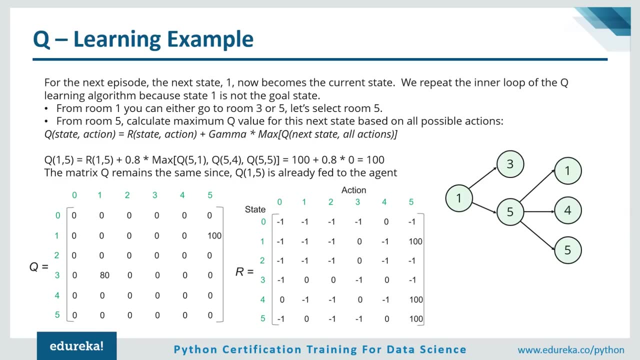 the maximum index, meaning that we're going to check which of the possible actions will give us the maximum Q value. all right, If you remember in our explanation over here, this value over here: max Q of five comma one, five comma four and five comma five. 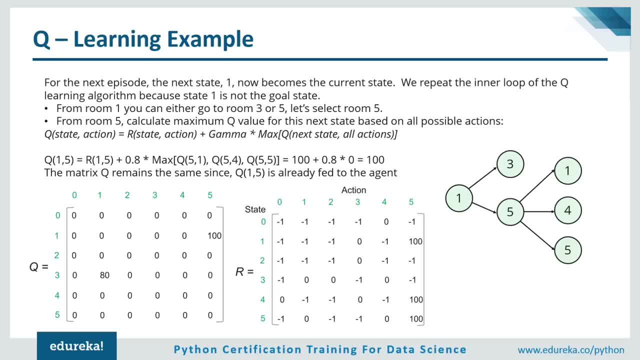 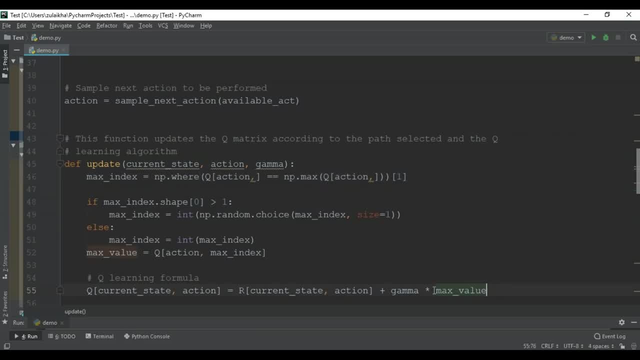 we had to choose a maximum Q value that we get from these three. So basically, that's exactly what we're doing in this line of code: We're calculating the index which gives us the maximum value. After we finish computing the value of Q, we'll just have to update our matrix. 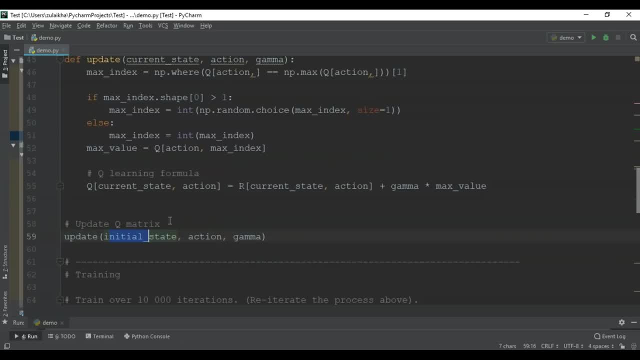 After that, we'll be updating the Q value and we'll be choosing a new initial state. okay, So this is the update function that is defined over here. Okay, so I've just called the function over here. So, guys, this whole set of code. 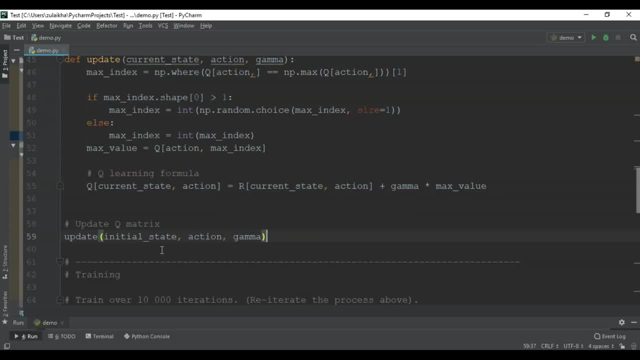 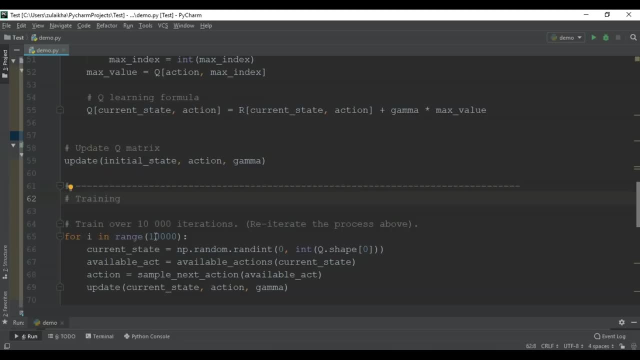 will just calculate the Q value. okay, This is exactly what we did in our examples. After that we have the training phase. So, guys, remember, the more you train an algorithm, the better it's going to learn. okay, So over here I've provided around 10,000 iterations. 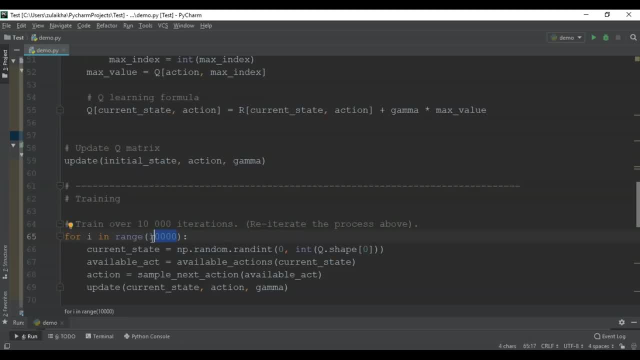 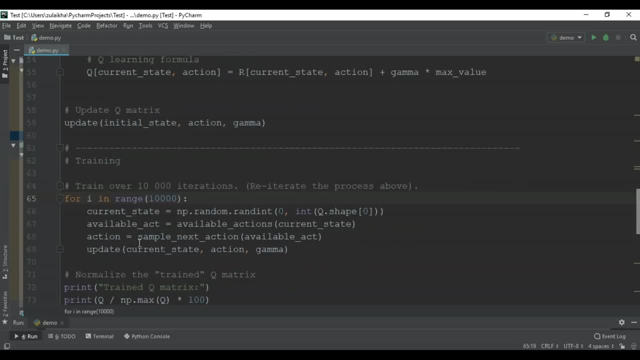 okay, So my range is 10,000 iterations, meaning that my agent will take 10,000 possible scenarios and it'll go through 10,000 iterations to find out the best policy. So here, exactly what I'm doing is I'm choosing the current state randomly. 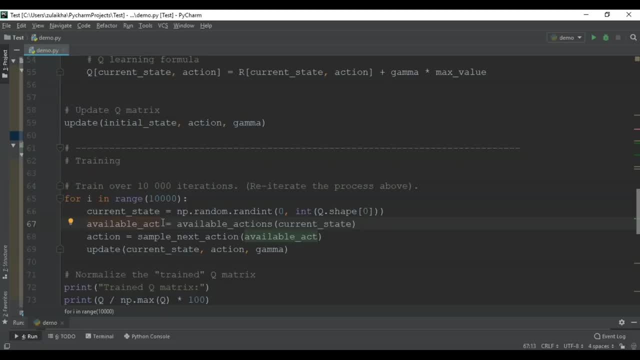 After that I'm choosing the available action from the current state, So either I can go to stage three or state five. Then I'm calculating the next action and then I'm finally updating the value in the Q matrix And next we just normalize the Q matrix. 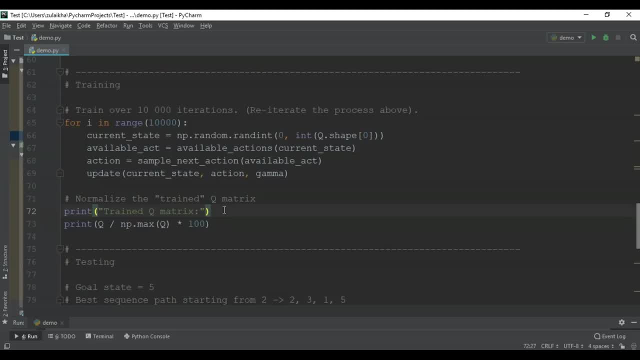 So sometimes in our Q matrix the value might exceed- okay, Let's say it exceeded to 500, 600. So that time you want to normalize the matrix, okay, We want to bring it down a little bit okay. 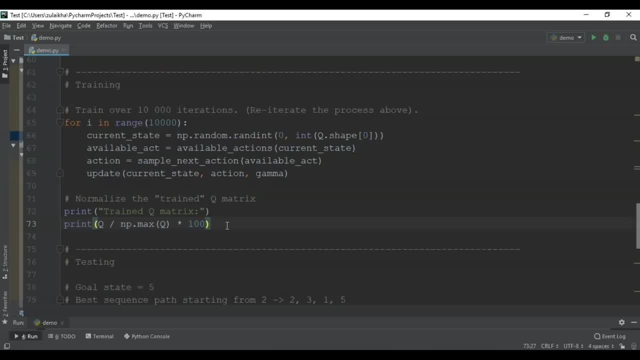 Because larger numbers we won't be able to understand And computation will be very hard on larger numbers. That's why we perform normalization. You're taking your calculated value and you're dividing it with the maximum Q value into 100.. All right, so you're normalizing it over here. 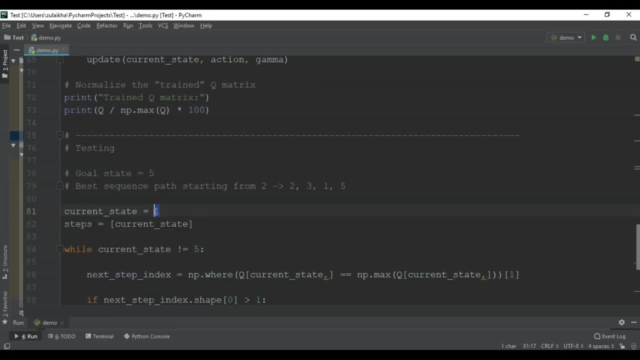 So, guys, this is the testing phase. okay, Here you'll just randomly set a current state and you won't give in any other data, because you've already trained a model. okay, You're going to give a current state, Then you're going to tell your agent that. 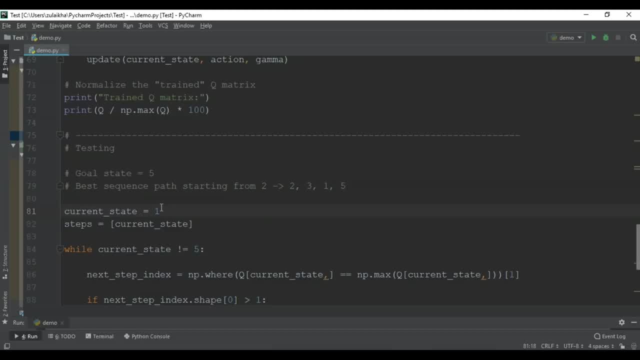 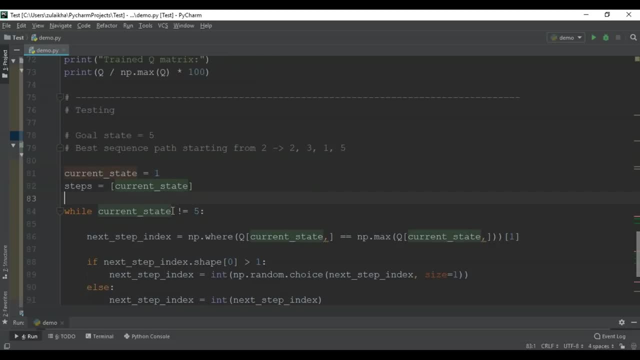 listen, you're in room number one. Now you need to go to room number five. okay, So he has to figure out how to go to room number five, because we've trained him now. all right, So here we've set the current state to one. 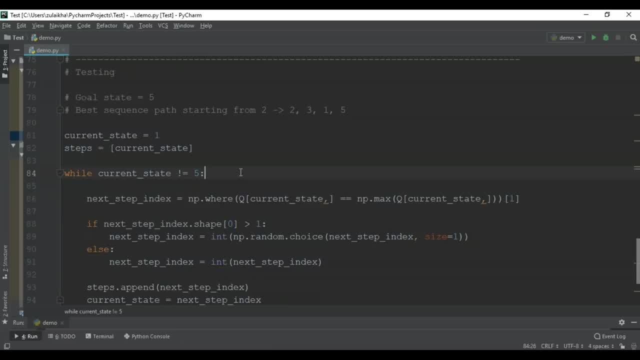 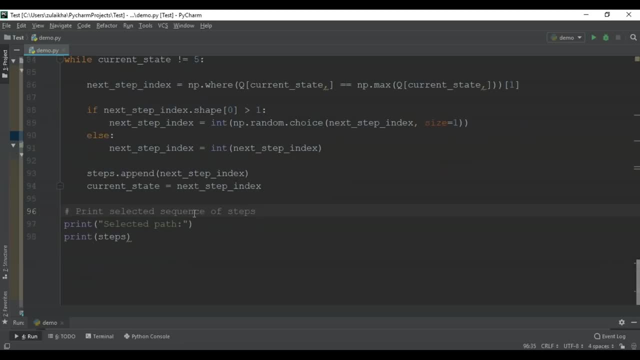 and we need to make sure that it's not equal to five, because five is the end goal. So, guys, this is the same loop that we executed earlier, So we're going to do the same iterations again. Now, if I run this entire code, 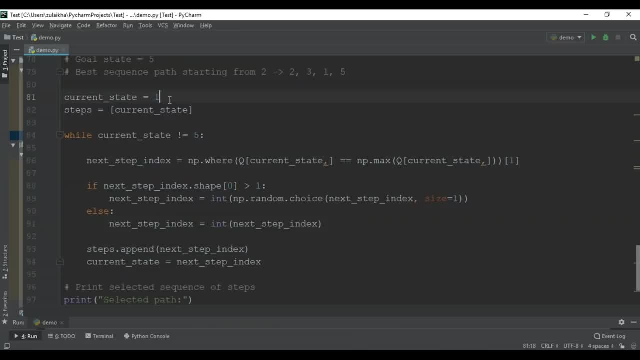 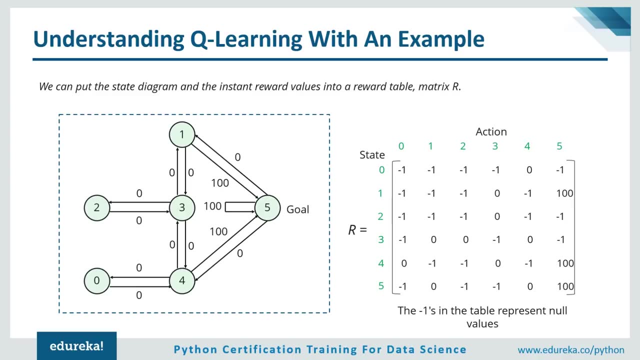 let's look at the result. So our current state here we've chosen as one okay, And if we go back to our matrix, you can see that there is a direct link from one to five, which means that the route that the agent should take. 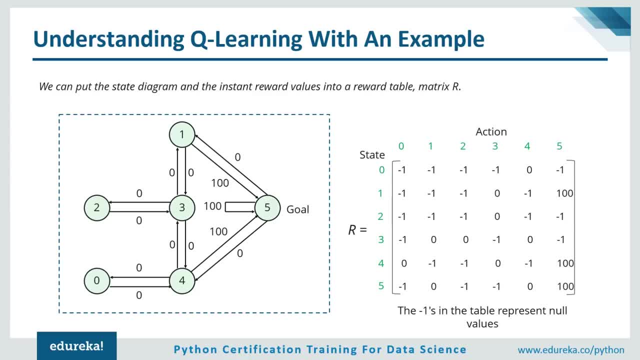 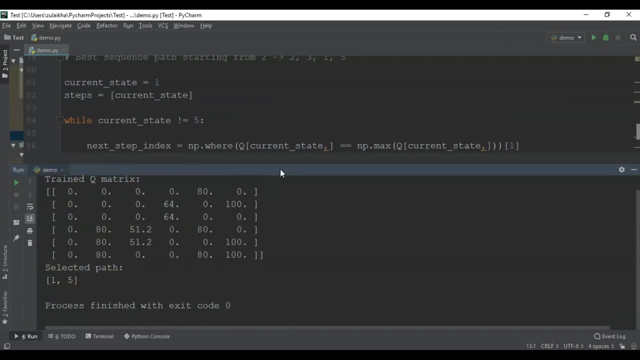 is one to five. okay, Directly it should go from one to five because it'll get the maximum reward, like that. Okay, let's see if that's happening. So if I run this, it should give me a direct path from one to five, okay. 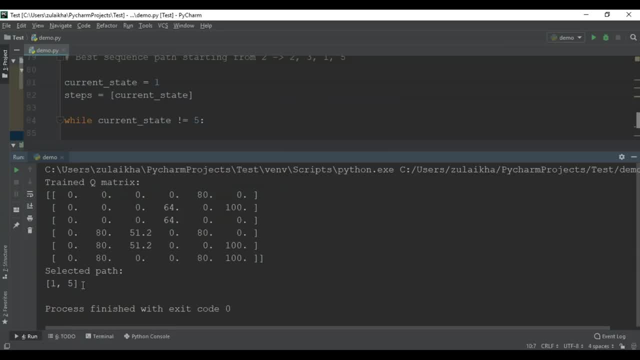 That's exactly what happened. So this is the selected path. So directly from one to five it went, and it calculated the entire queue matrix for me. So, guys, this is exactly how it works. Now let's try to set the initial stage as, let's say, two. 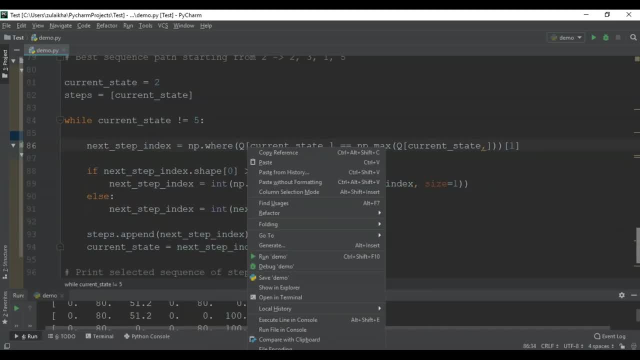 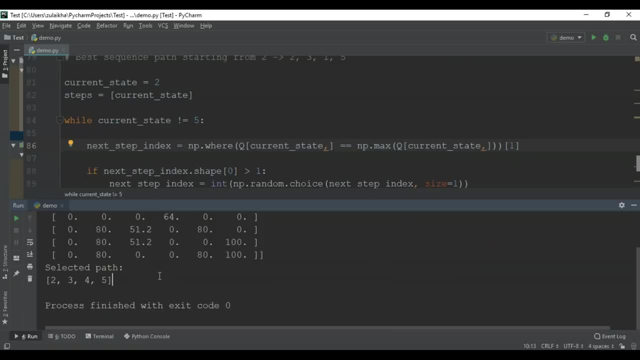 So if I set the initial stage as two and if I try to run the code, let's see the path that it gives. So the selected path is two, three, four, five. Now it chose this path because it's giving us the maximum reward from this path. okay, 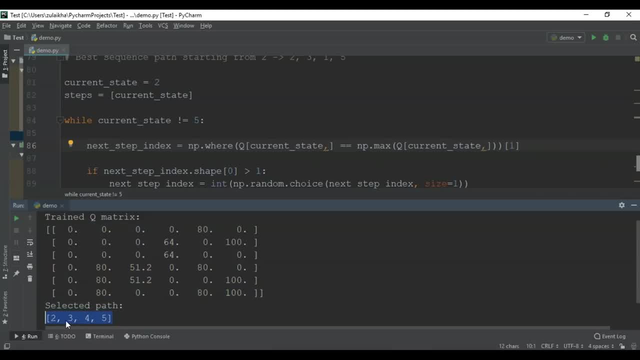 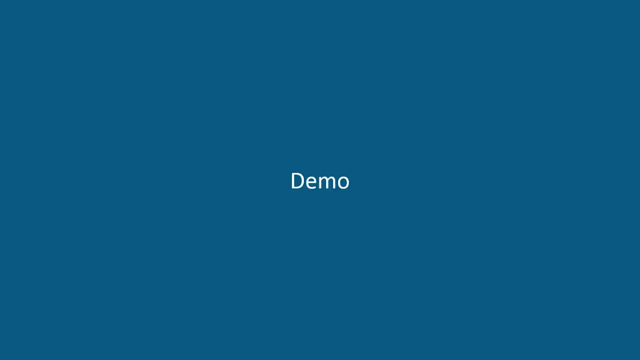 This is the queue matrix that it calculated And this is the selected path. All right, so, guys, with this we come to the end of this demo. So, basically, what we did was we just placed an agent in a room- random room- and we asked it to traverse through. 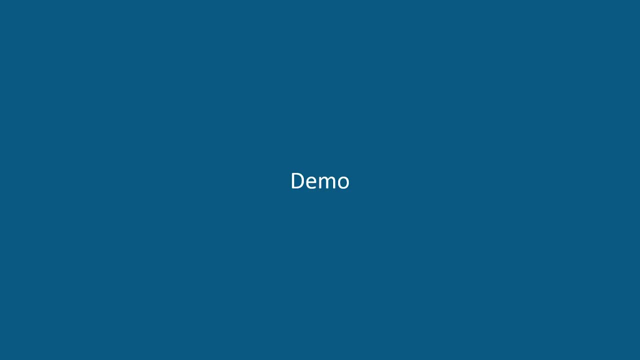 and reach to the end room, which is room number five. So, basically, we trained our agent and we made sure that it went through all the possible paths to calculate the best path. all right, So, guys, with this we come to the end of today's demo.